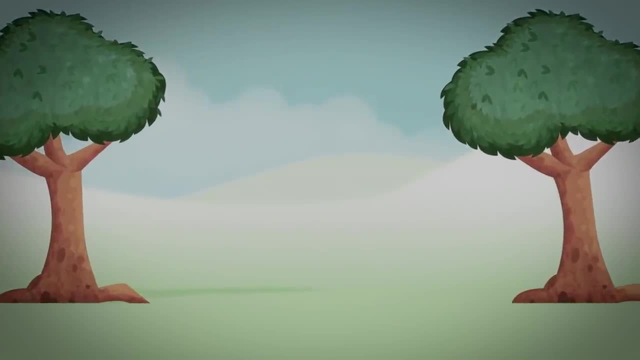 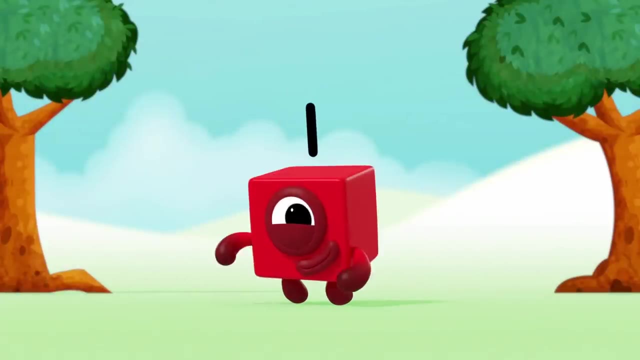 If there's nothing going on, no one's there and it's no fun. you can get the party started with a bang by adding one. I am one and I'm playing in the sun. Being one is my idea of fun. One, One little block. 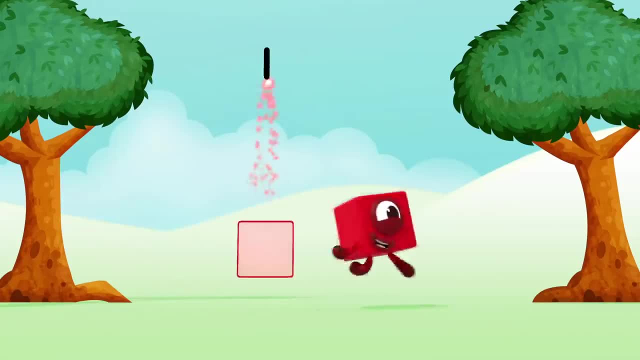 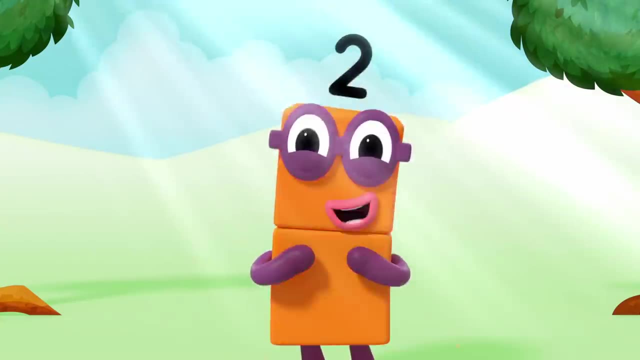 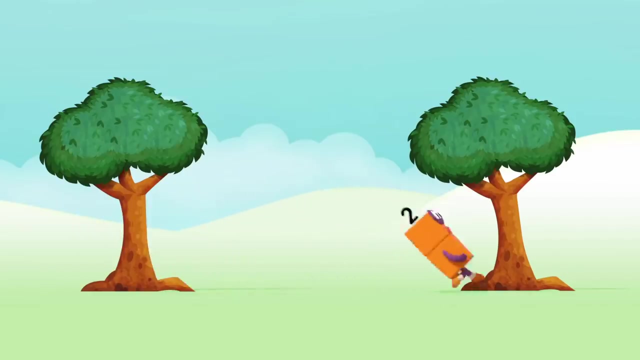 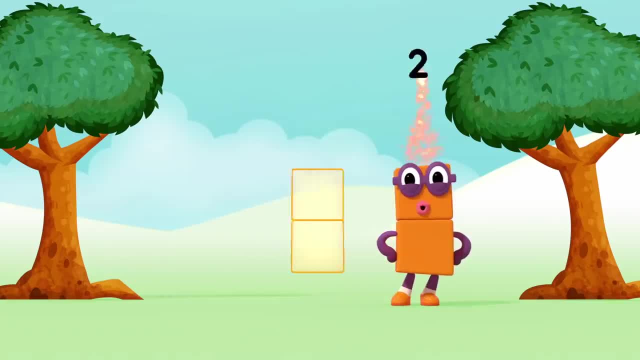 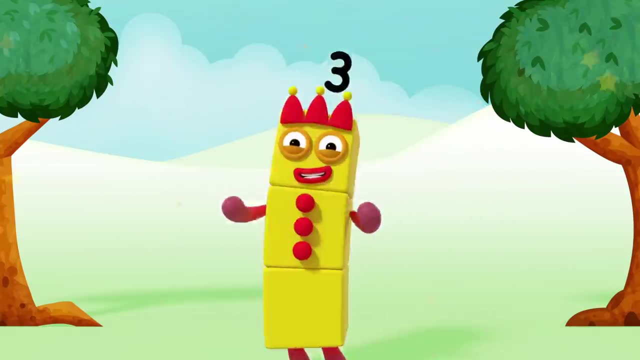 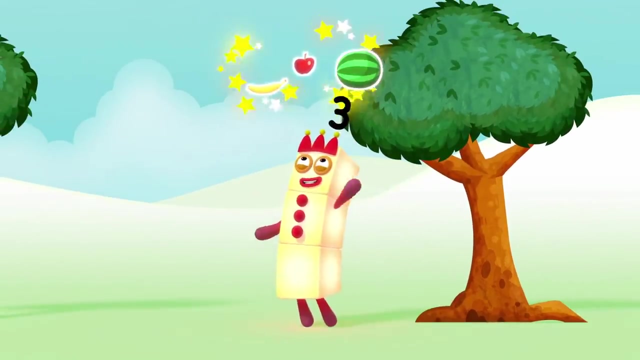 Now let's add another one. Two plus one equals three. I am three and I'm playing in the sun. Juggling things is my idea of fun. One, two, three, Three things. Look at me: One, two, three. 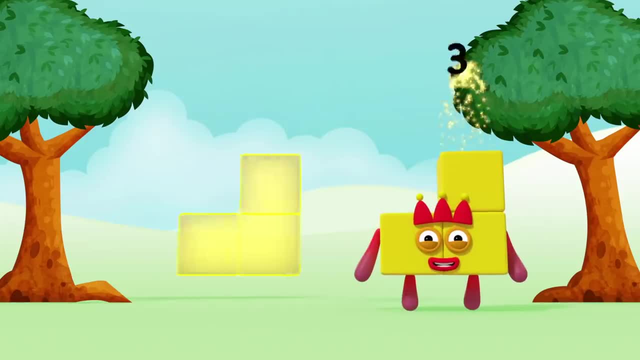 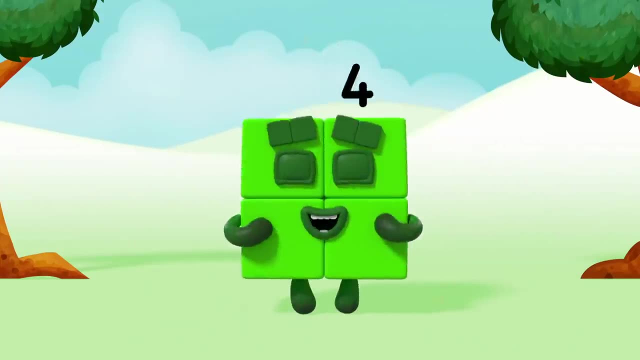 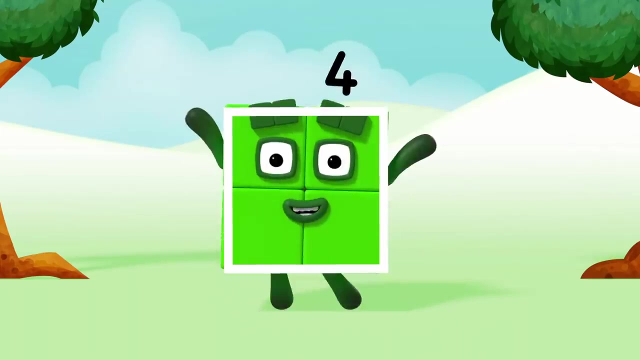 Now let's add another one. Three plus one equals four. I am four and I'm playing in the sun. Being square is my idea of fun. One, two, three, four, Four sides. Ouch, ouch, ouch, ouch. 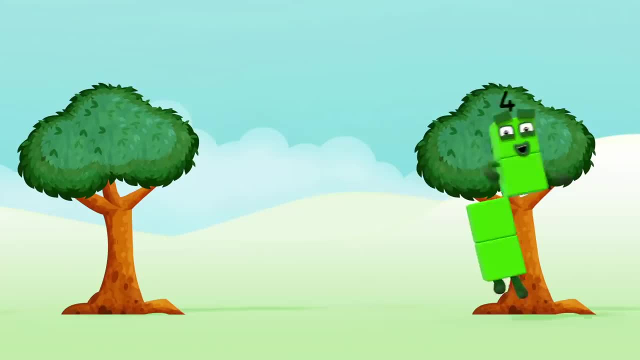 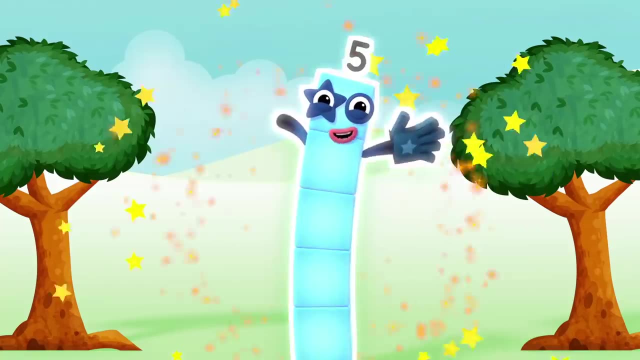 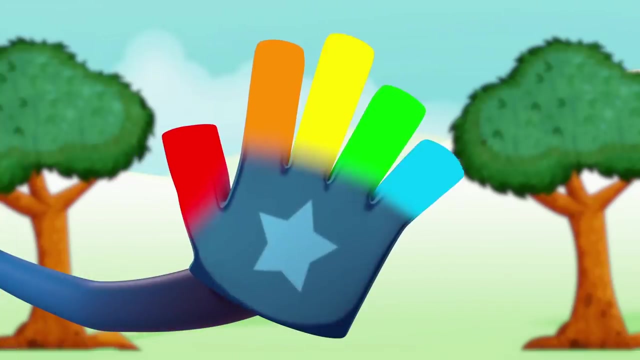 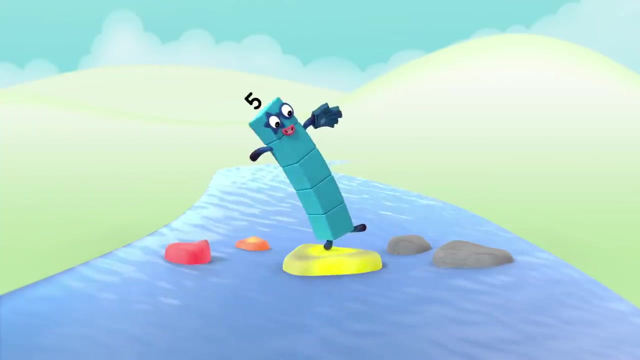 Four corners. Now let's add another one. Four plus one equals five. I am five and I'm playing in the sun. High five are my idea of fun: One, two, three, four, five, Five fingers. If you add another one, the number gets one bigger. 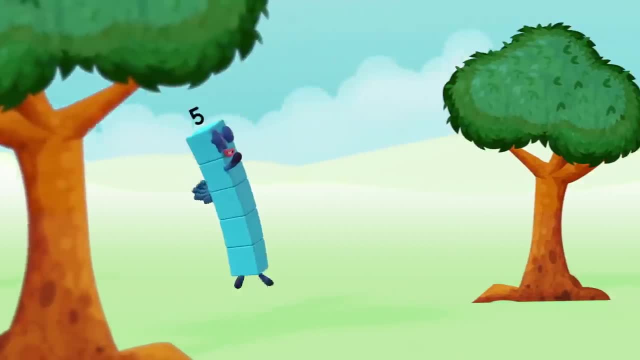 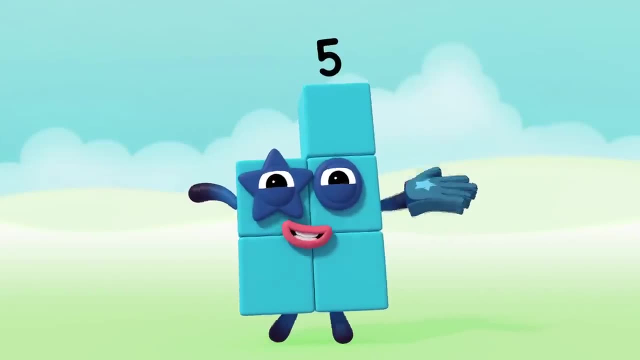 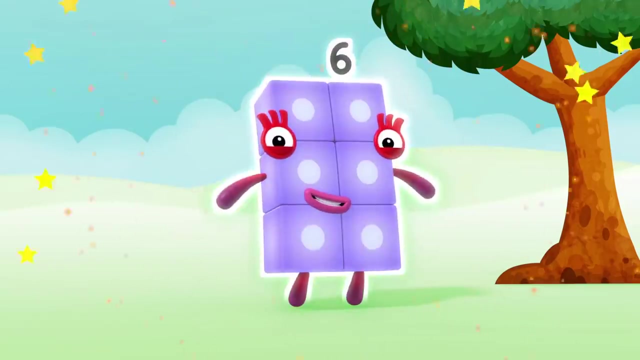 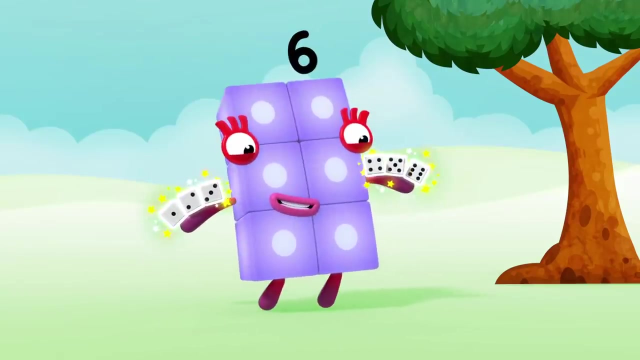 And if you keep on adding one you can get to any bigger. Now let's add another one. Five plus one equals six. I am six and I'm playing in the sun. Playing games is my idea of fun. One, two, three, four, five, six. 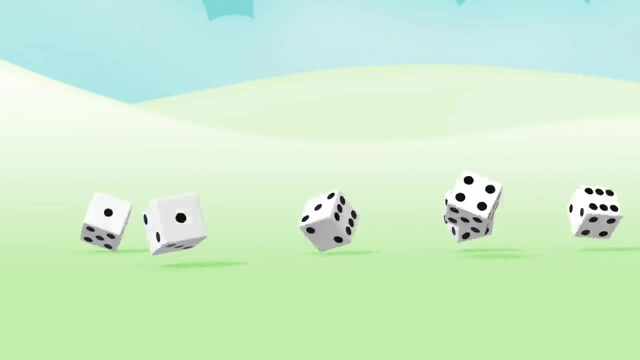 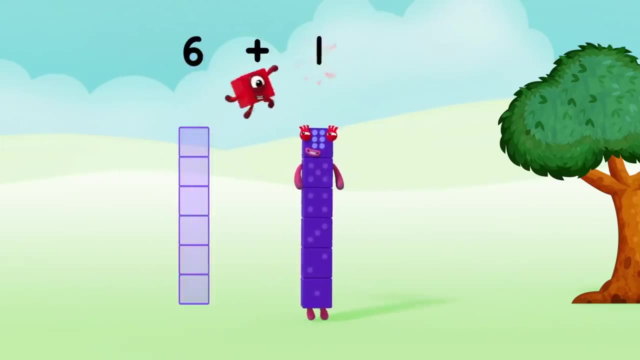 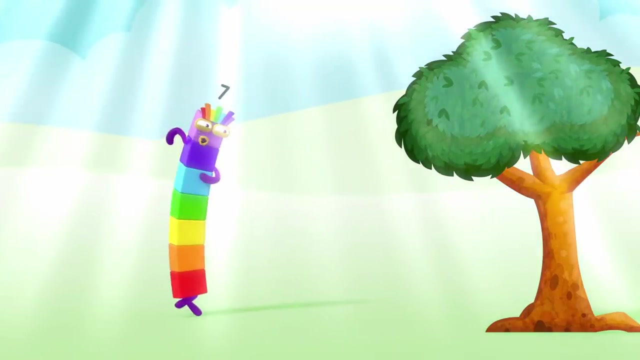 Six dice. Now let's add another one. Six plus one equals seven. I am seven and I'm playing in the sun. Making rainbows is my idea of fun. One, two, three, four, five, six, seven. 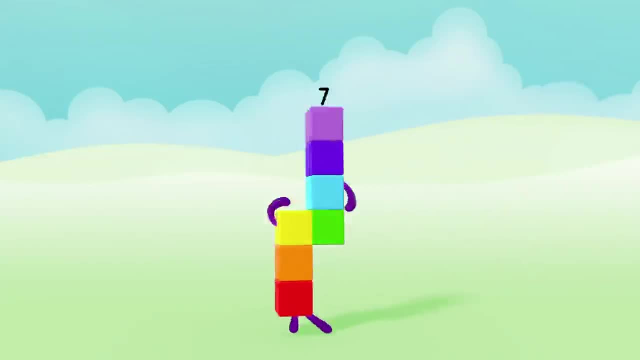 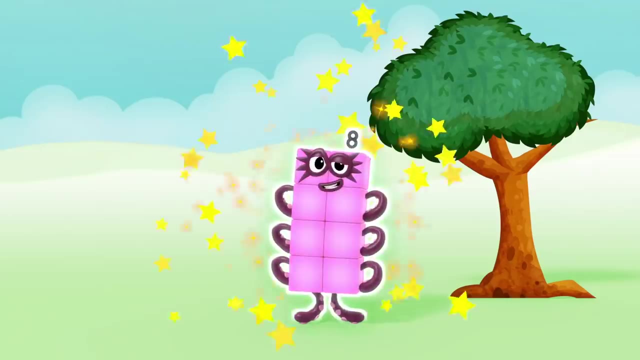 Seven colors. Now let's add another one. Seven plus one equals eight. I am eight and I'm playing in the sun, And I'm playing in the sun. being Octoblock Is my idea of fun Octoblock run. 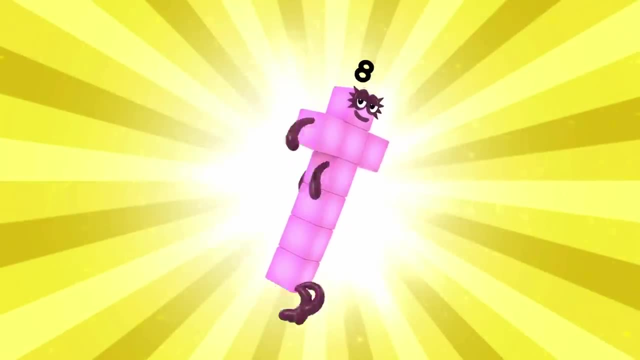 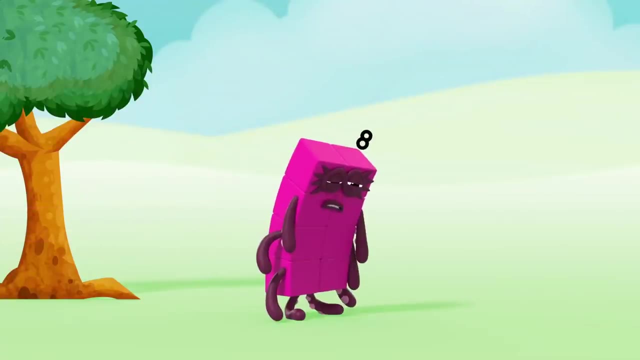 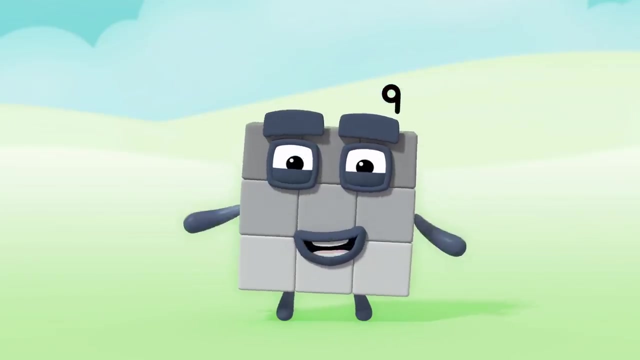 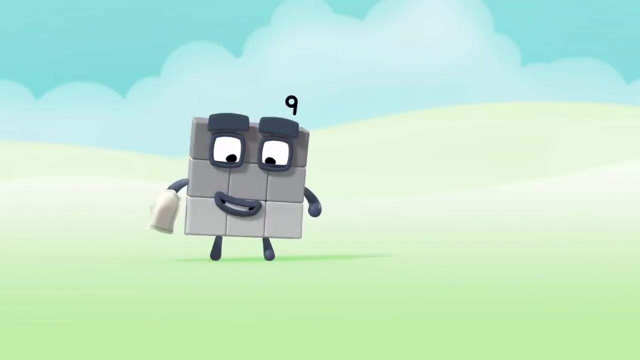 One, two, three, four, five, six, seven, eight Run. Now let's add another one. Eight Plus one equals nine. I am nine, Ten, I am nine and I'm playing in the sun. Not sneezing is my idea of fun. 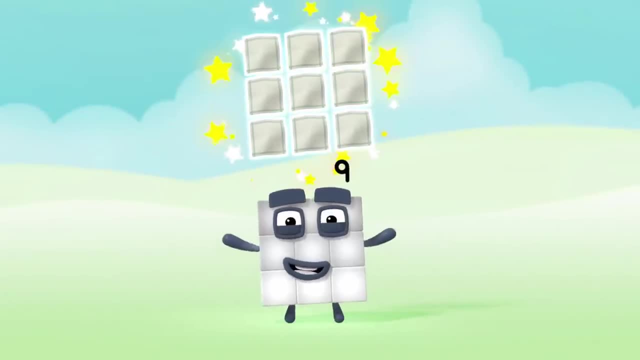 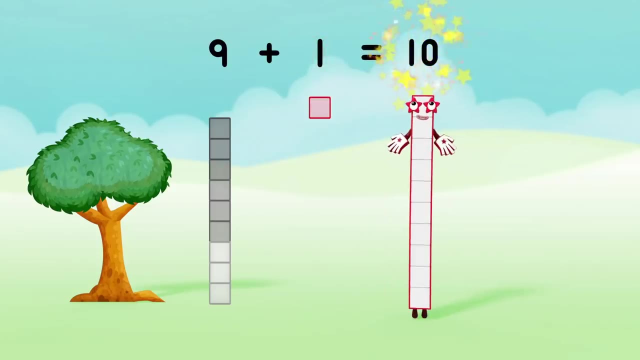 One, two, three, four, five, six, seven, eight, nine, Nine hankies. Now let's add another one. Nine plus one equals ten. I am ten and I'm playing in the sun. Being ten is my idea of fun. 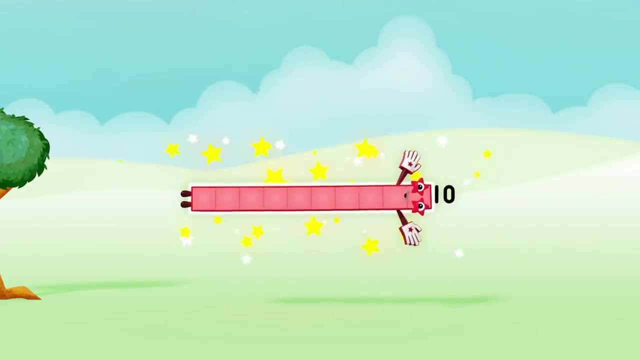 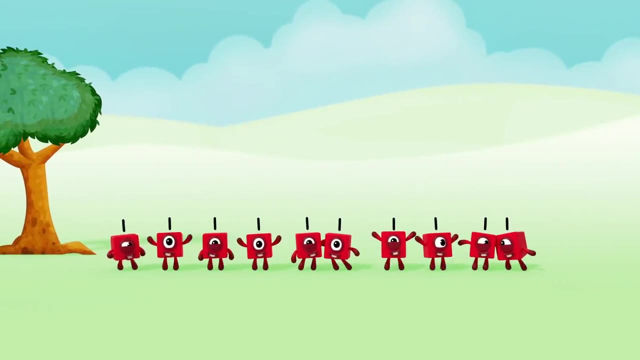 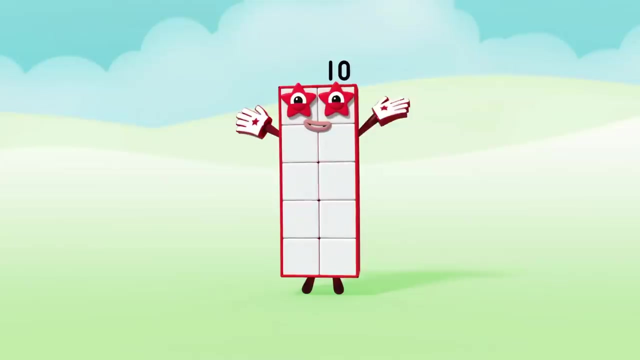 One, two, three, four, five, six, seven, eight, nine, ten, Ten blocks. We're ten ones And we're playing in the sun. Making friends is our idea of fun. One, two, three, four, five, six, seven, eight, nine, ten. 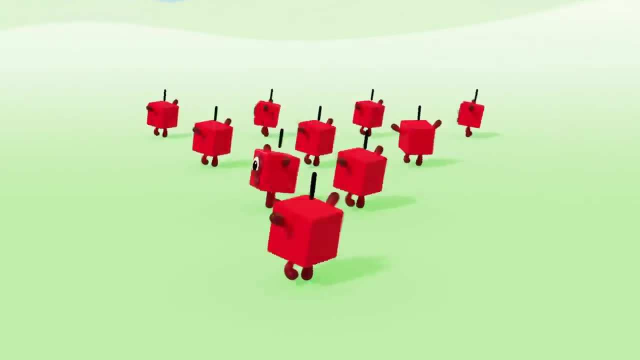 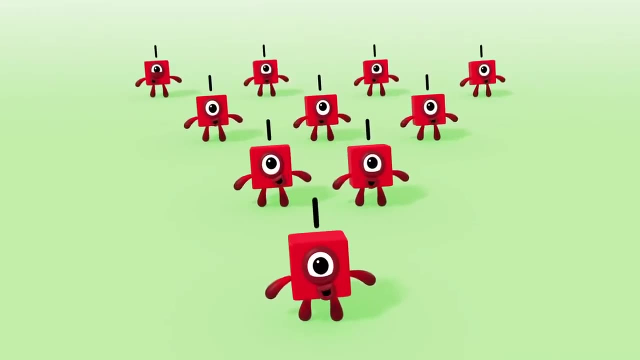 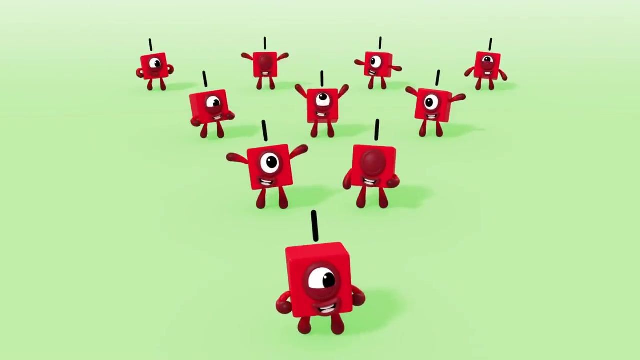 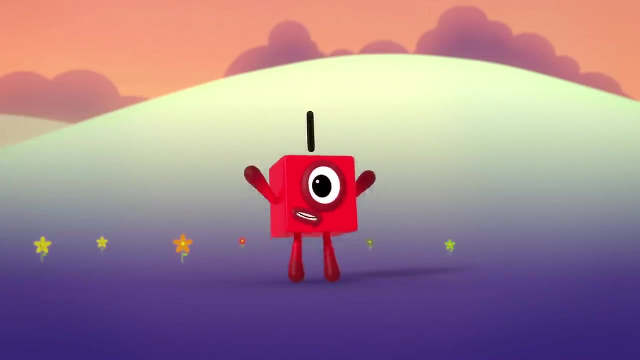 Remember this forever. You can do what we've just done. You can make any number. Then you keep on adding one. That was fun. Yay, I'm number one, And this is fun. I've got one block to play with and the whole of me is one. 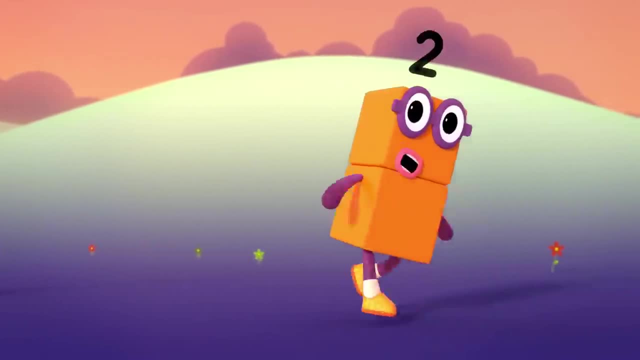 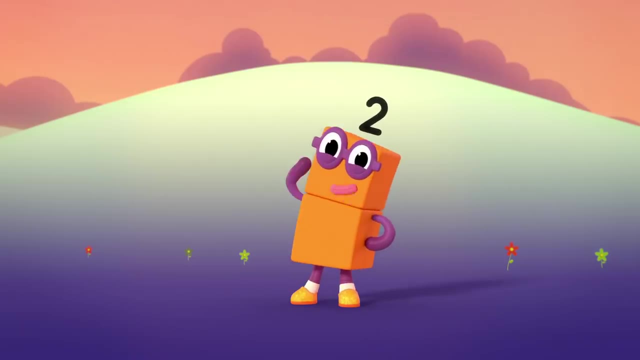 One, One, two, one, two. I'm number two. How do you do? I've got two blocks to play with and the whole of me is two. One, two. Now I'm number three. One is a part of me and one is a part of me and the whole of me is two. 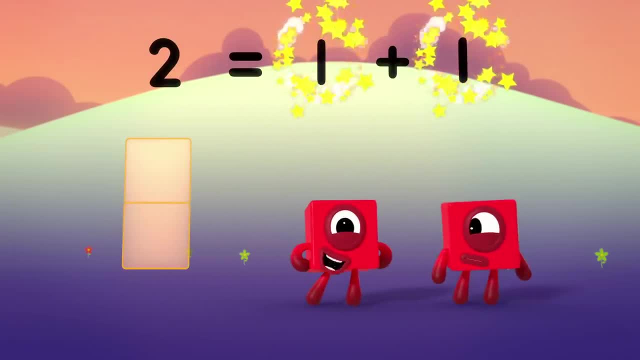 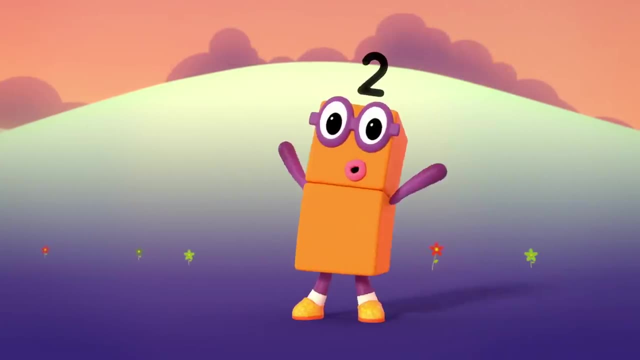 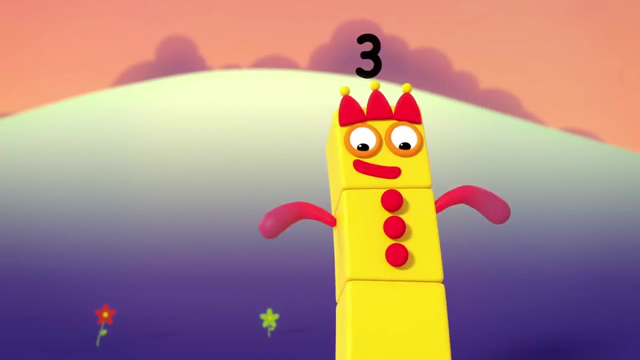 Watch. I'm one and I'm a part, I'm one and I'm a part, And the whole of me is two, One, two, three, One, two, three, One, two, three. I'm number three. 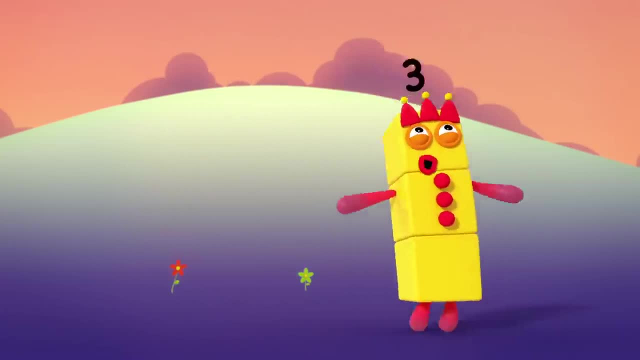 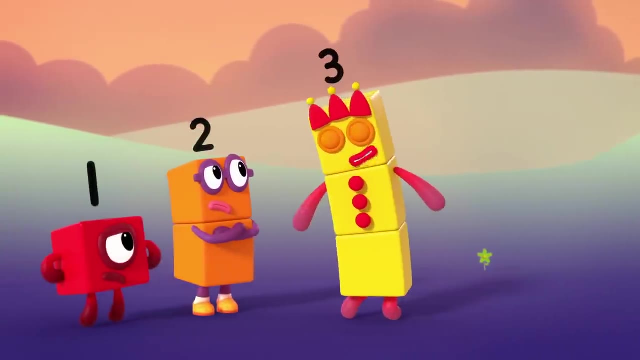 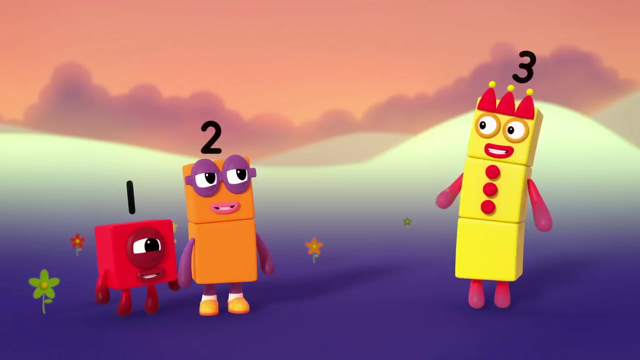 I'm the best of all the number blocks, as you can plainly see. The whole of me is amazing. The whole of me is so great. The whole of me is Sorry. Three, Try again. OK, I'm number three. Yes, look at me. 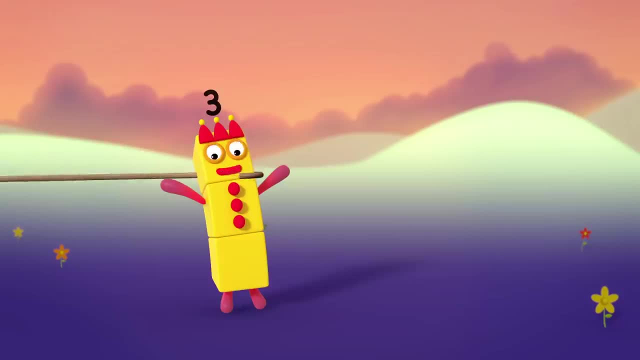 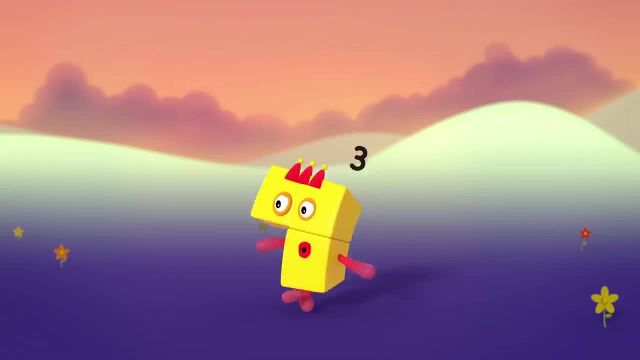 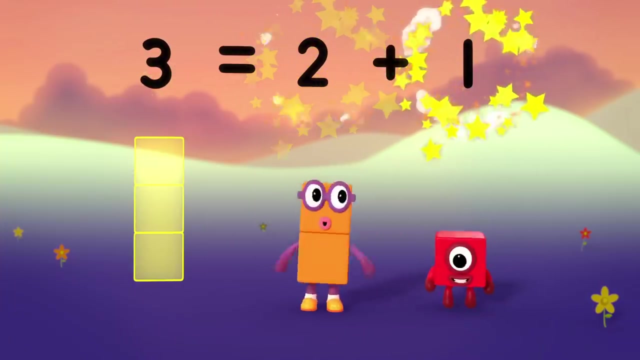 Now look at me. I've got three blocks to play with, And the whole of me is three. One, two, three. One is a part of me And two is a part of me, And the whole of me is three. What I'm two and I'm a part. 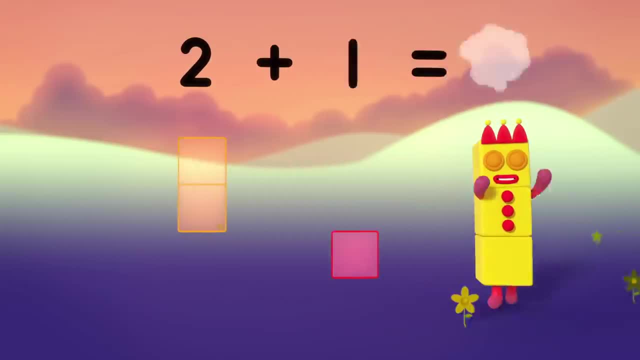 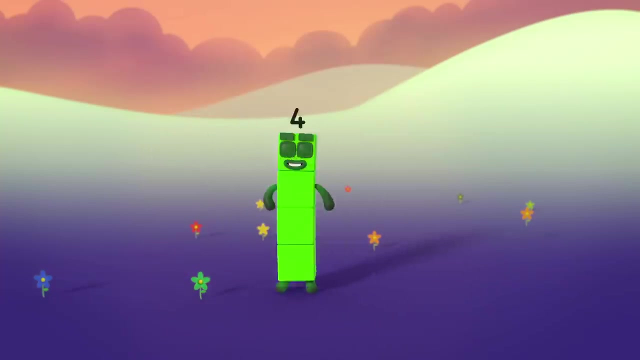 I'm one and I'm a part, And the whole of me is three. One, two, three. I'm number four And I am sure That I've got four blocks to play with, And the whole of me is four. One, two, three, four. 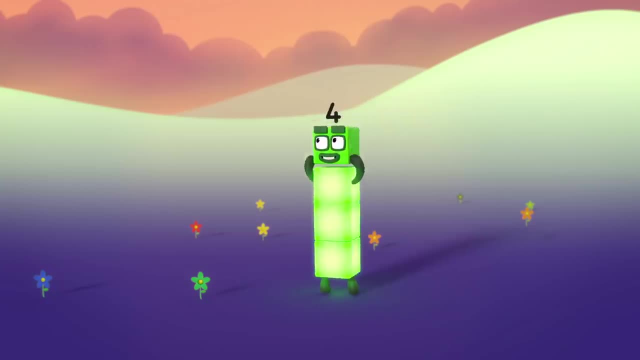 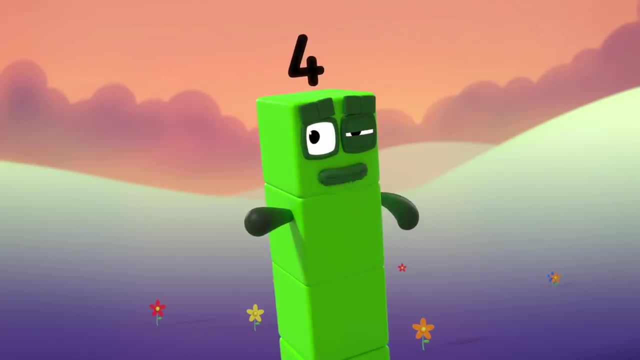 One is a part of me And three is a part of me And the whole of me is four. What I'm three and I'm a part. I'm one and I'm a part And the whole of me is four. Now, here is something more That's different from before. 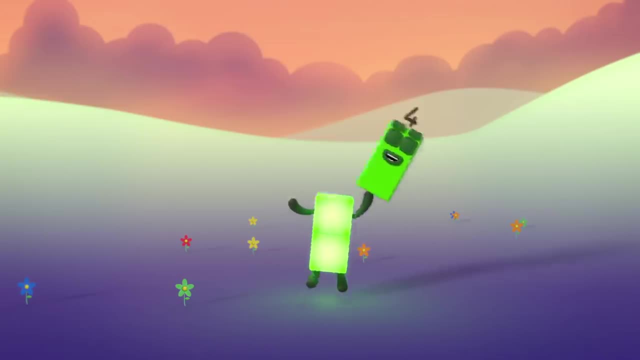 Two is a part of me, And two is a part of me And the whole of me is four. What I'm two and I'm a part. I'm two and I'm a part And the whole of me is four. I'm a square, look. 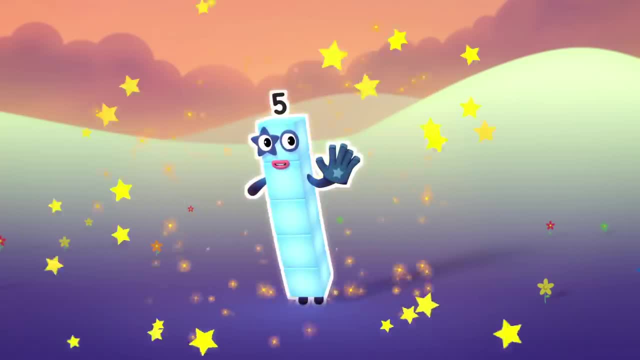 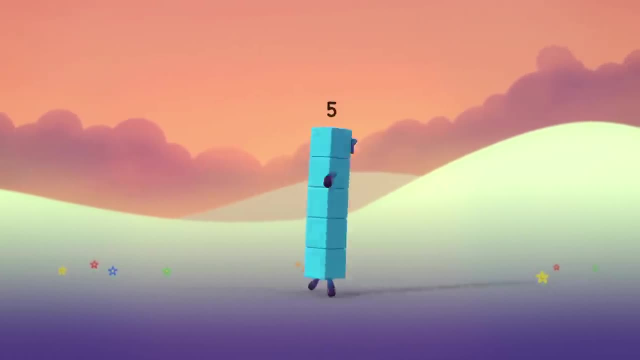 Four sides, four corners. I'm number five, I am alive, I've got five blocks to play with And the whole of me is five. One, two, three, four, five. One is a part of me And four is a part of me. 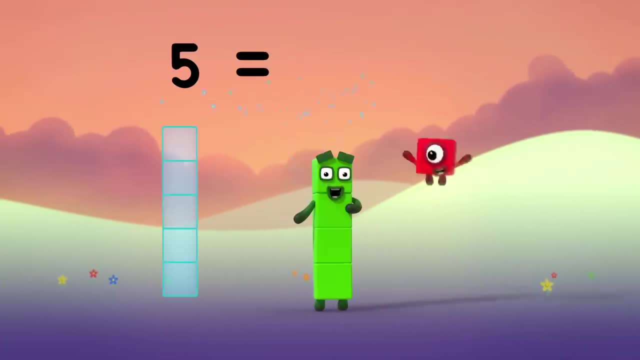 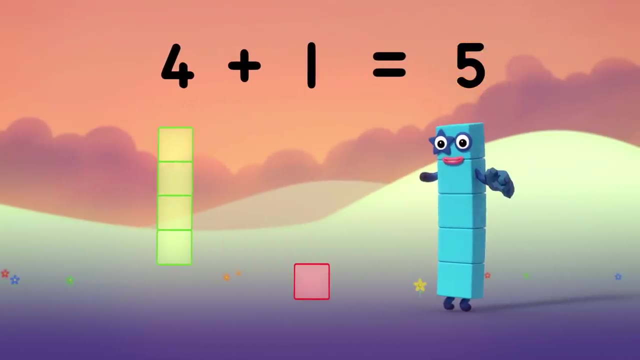 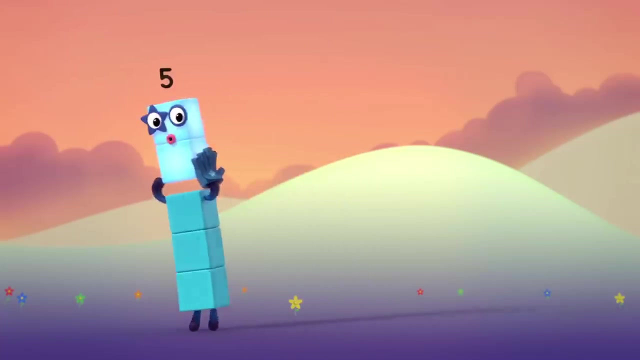 And the whole of me is five. What I'm four and I'm a part. I'm one and I'm a part And the whole of me is five. But now I feel alive going into overdrive. Two is a part of me And three is a part of me. 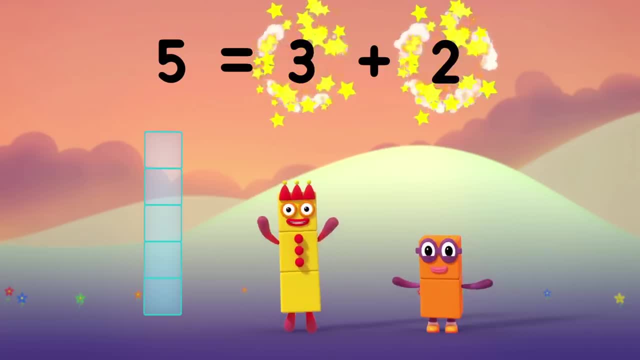 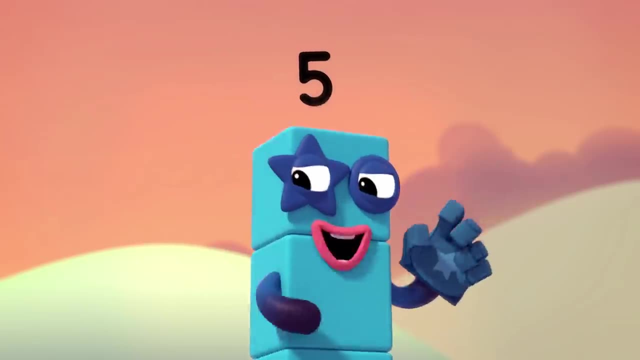 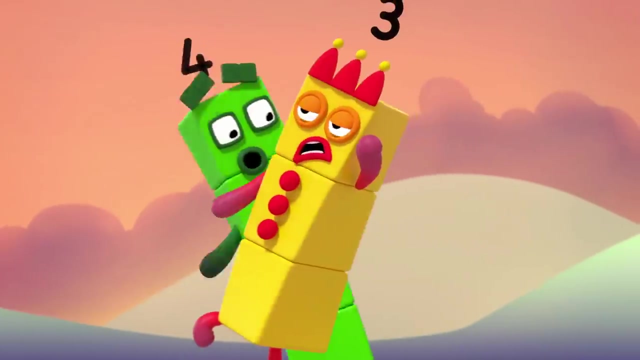 And the whole of me is five. One and three and I'm a part, I'm two and I'm a part, And the whole of me is five High five. Making friends is easy when you can come apart. Splitting up is not so hard. it won't break your heart. 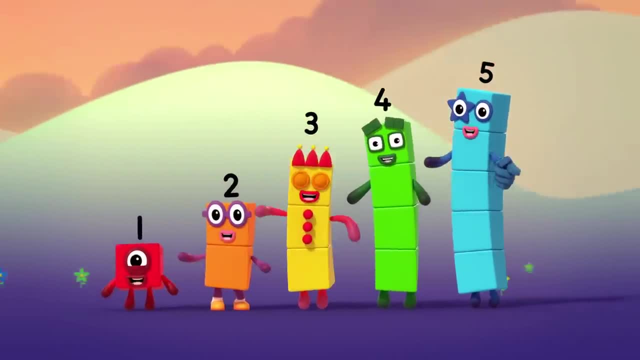 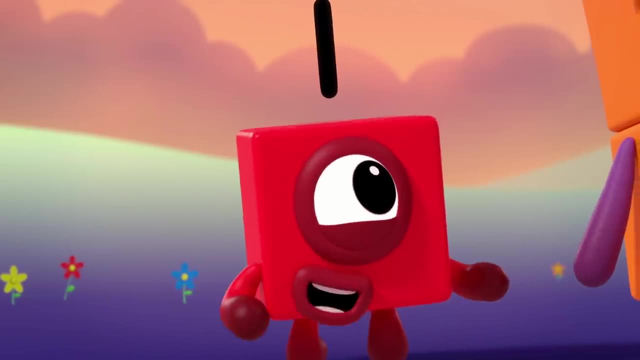 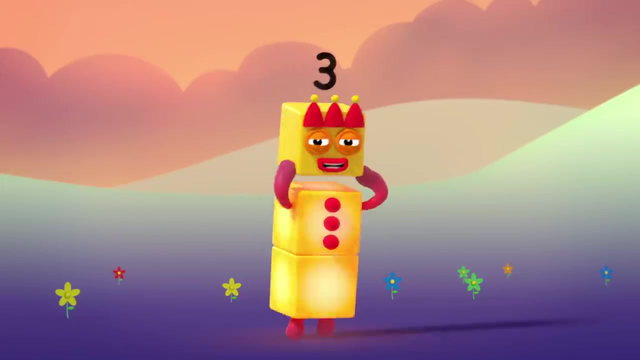 So when we fall to pieces, We have lost control. A whole is made of all its parts And the parts they make a whole. Just remember that One is a part of me And one is a part of me. One is a part of me And two is a part of me. 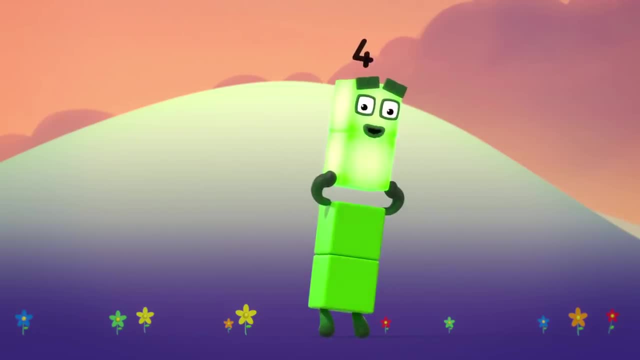 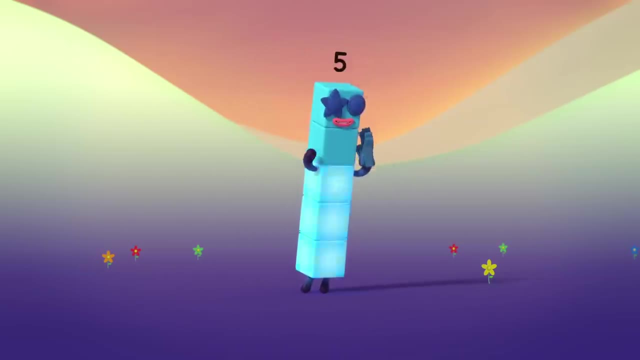 One is a part of me And three is a part of me. Two is a part of me And two is a part of me. One is a part of me And four is a part of me. Two is a part of me And three is a part of me. 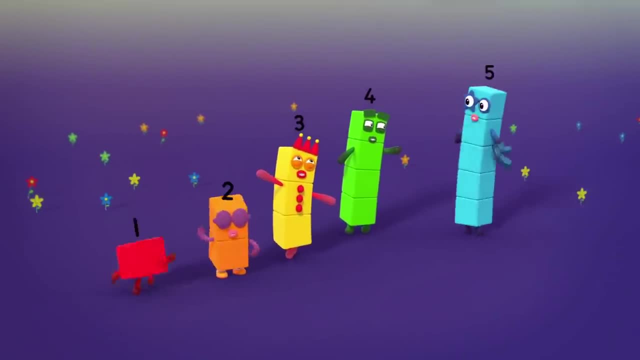 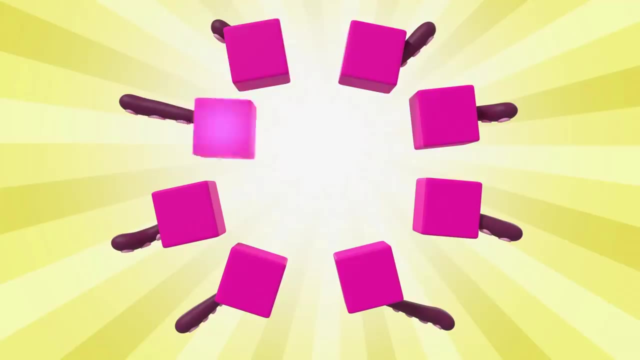 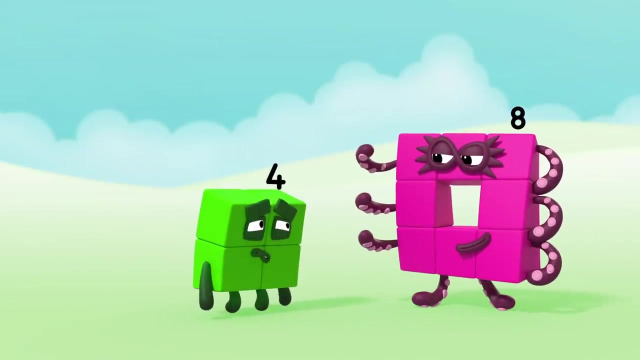 And the whole, The whole of me is one, two, three, four, five. One, two, three, four, five, six, seven, eight. Rearrange, How's this? Um, you're a square with a With a hole. 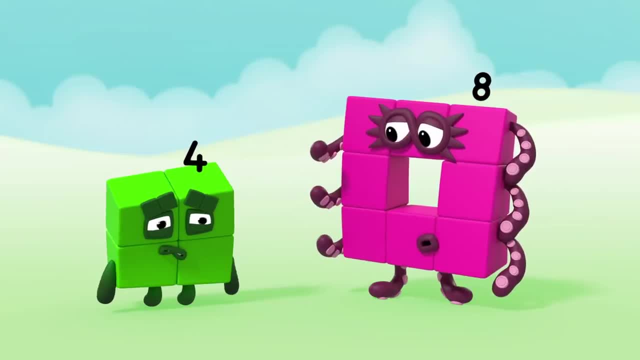 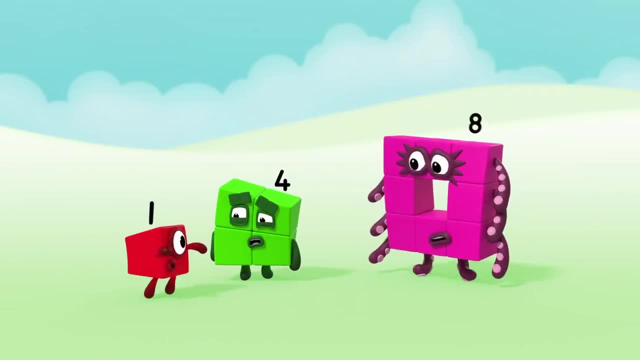 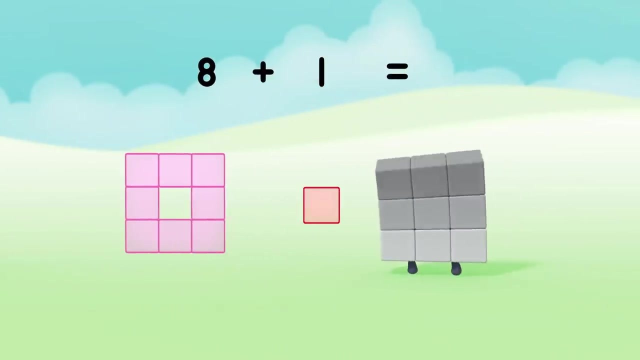 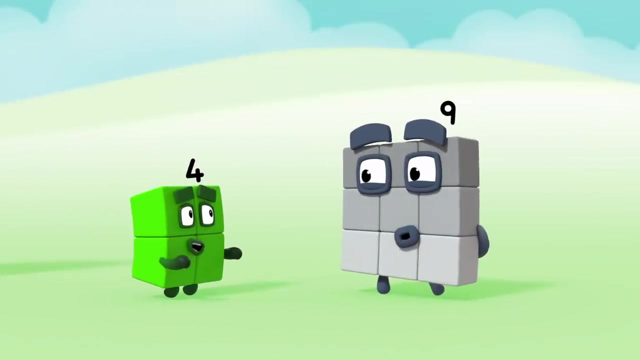 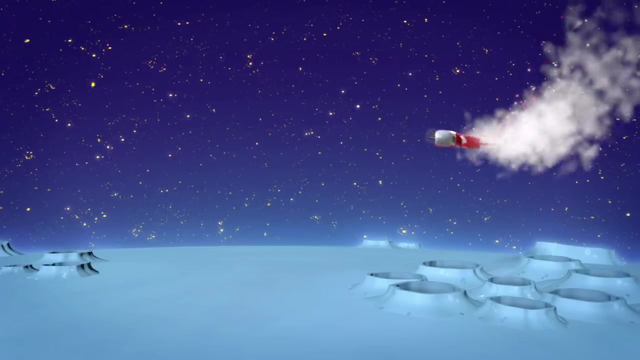 That doesn't really count. Oh, I'm sorry for Hole, me, Me Hole, Look. Hmm, Eight Plus one Equals Nine. I am nine And I feel fine. Square, Hello, Big square, Number ten up on the moon. 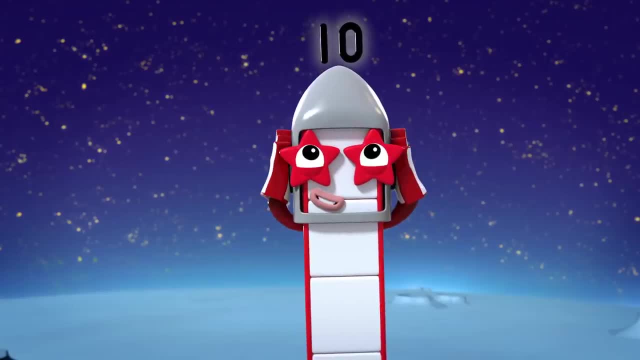 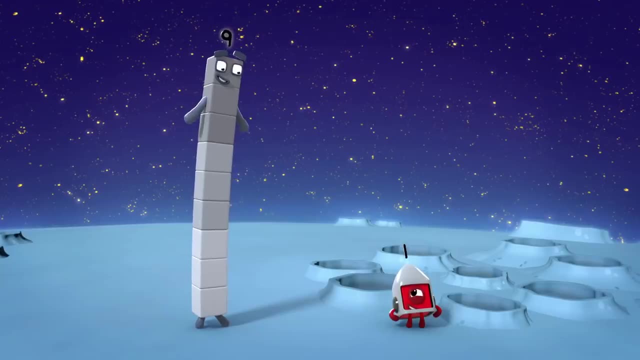 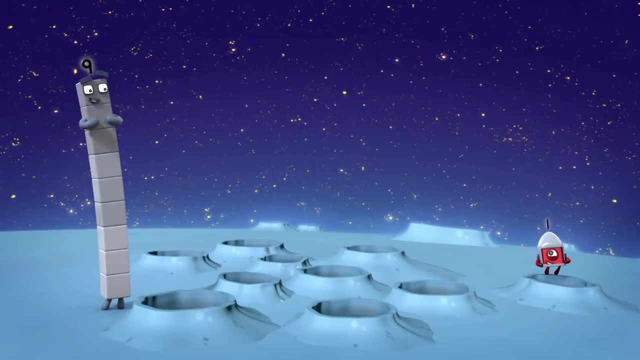 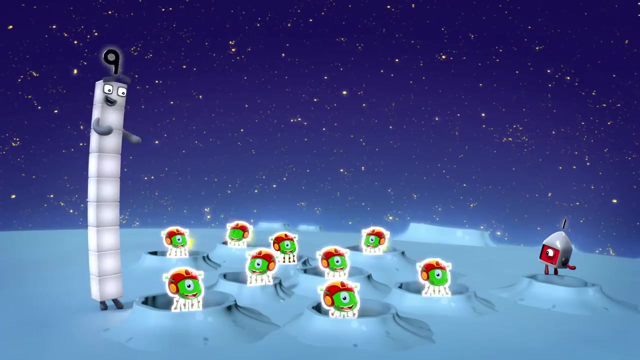 And my friends will be Here soon. Ten equals Nine Plus one. One small step for a number, One giant hop for number kind, We're on the moon. Nine And one. That was easy. This is fun. One, two, three, four, five, six, seven, eight, nine. 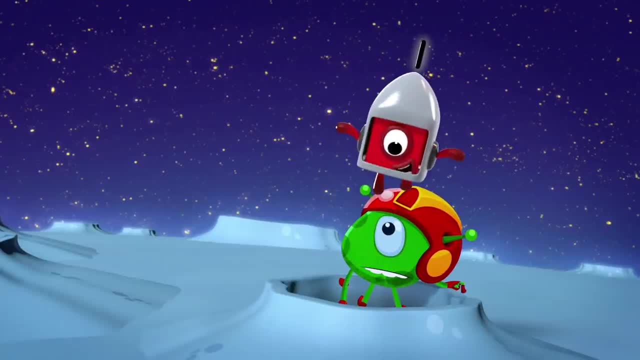 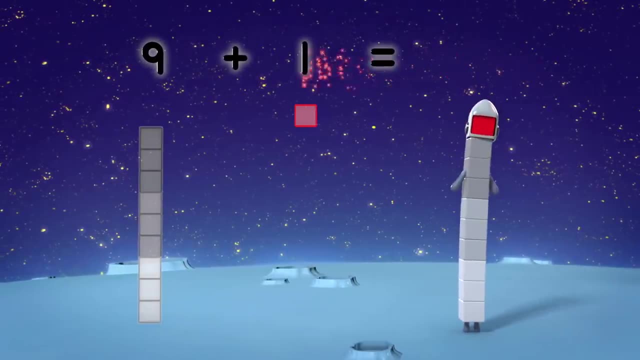 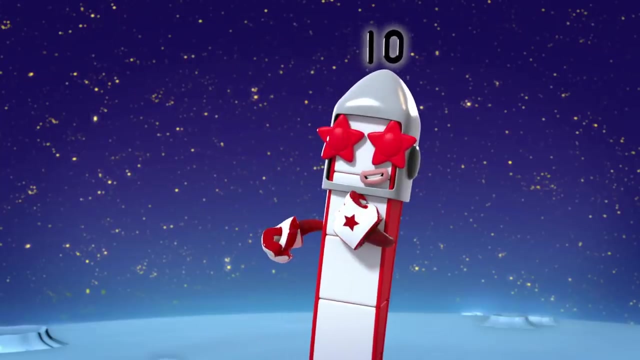 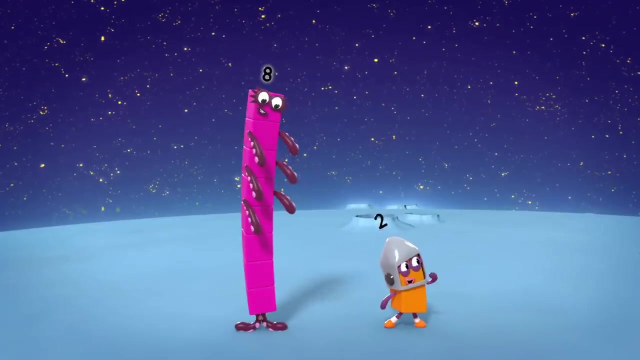 Nine aliens And one more is ten. Whoa, Nine Plus one Equals ten. Number ten back on the moon. Two more friends will be here soon. Ten equals Eight Plus two. We're on the moon Eight. 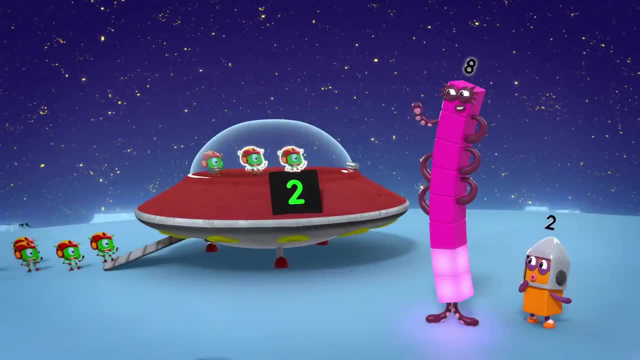 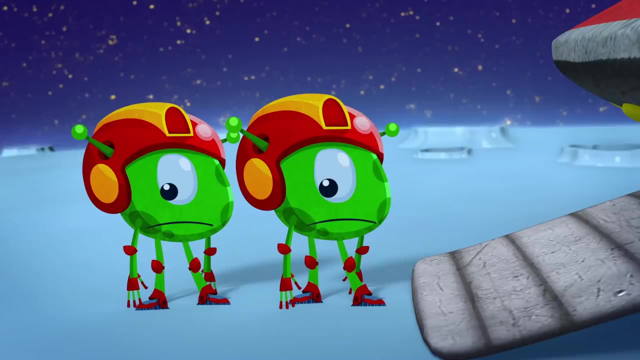 And two. How did we get here? Haven't a clue? One, two, three, four, five, six, seven, eight, Eight aliens All heading home. Oh no, There's no room for those two, Never fear. 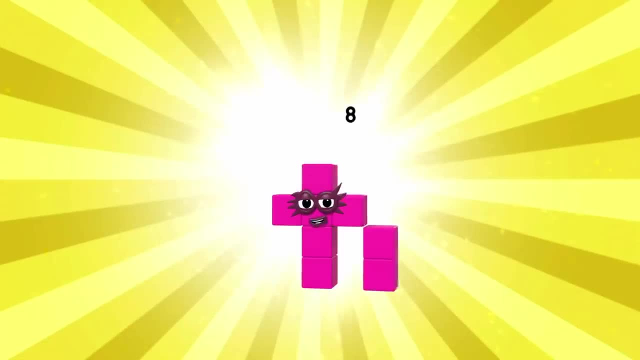 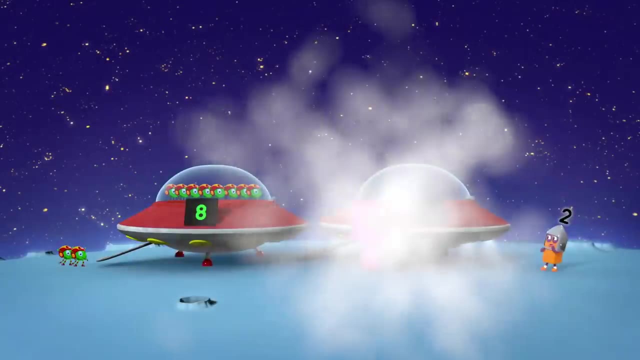 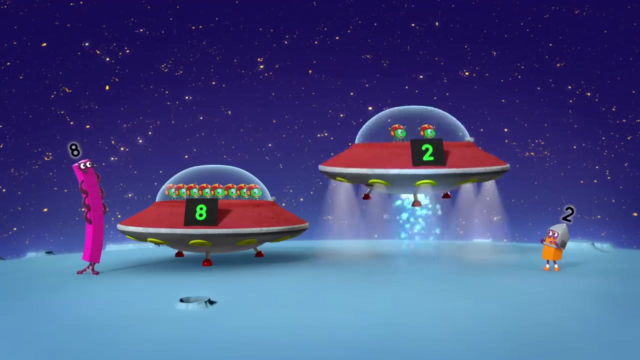 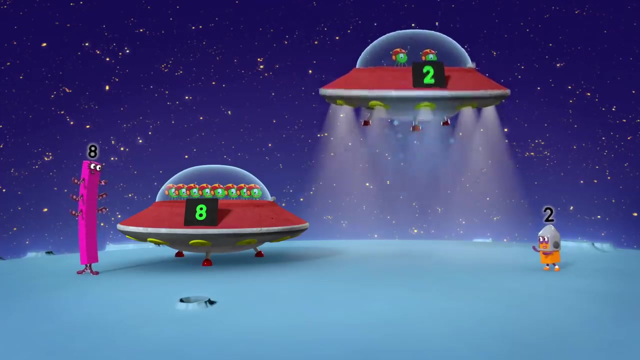 Octoblock is here. Octoblock: Bill One, two, three, four, five, six, seven, eight. Bill Two: flying saucers. Good work. Oh, come back, It's not starting, Whoa. 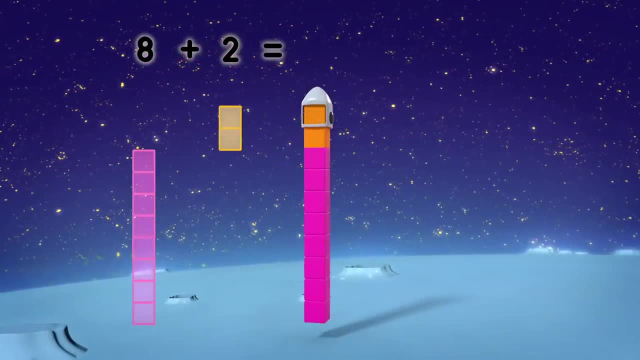 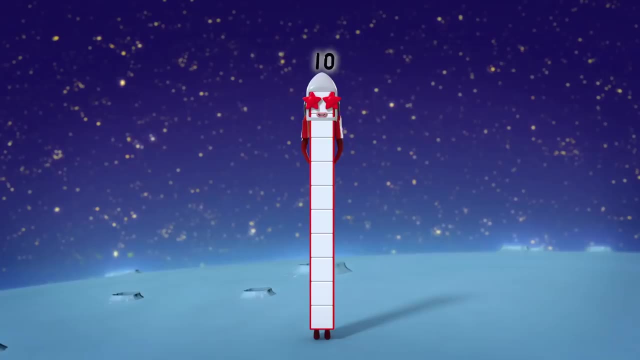 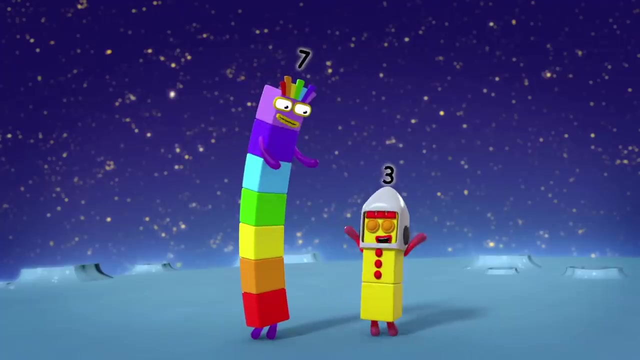 Eight plus two equals Ten. Here I am, number ten Time to make some friends again. Ten equals seven plus three. We're on the moon. Seven and three, We're so lucky. Look at me, Woo-hoo, Look at that. 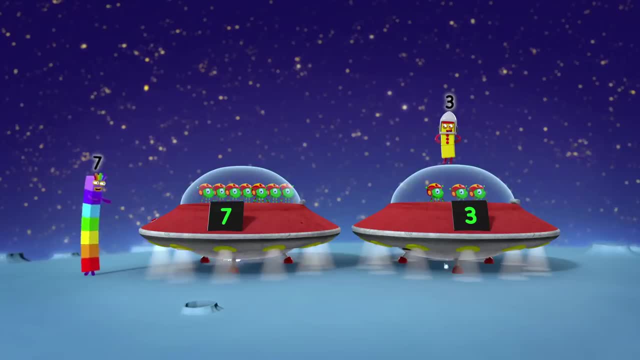 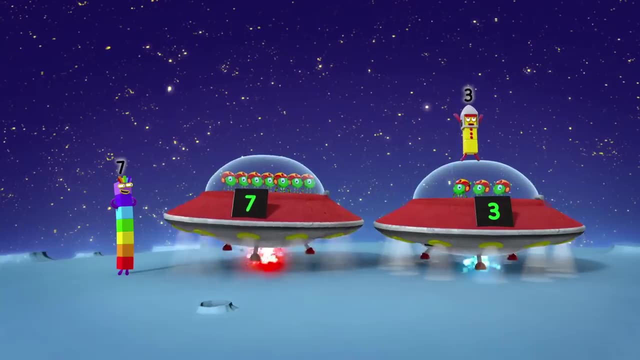 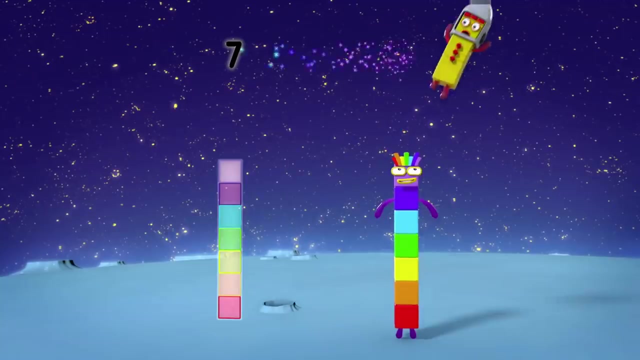 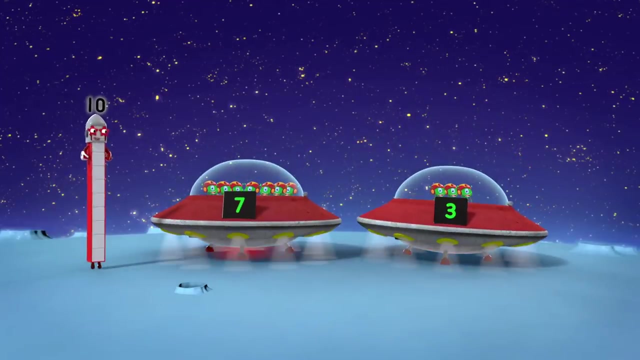 There's the on button. That was lucky. Ooh, Ready, steady, Blast off. Ugh, It's too heavy, Ha-ah. Seven plus three equals ten. It's ten again. Wait and see who my next two friends will be. 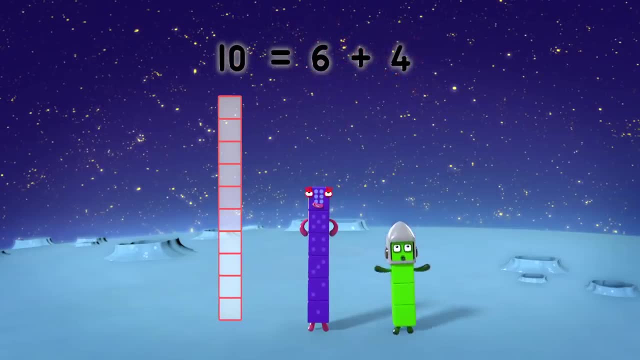 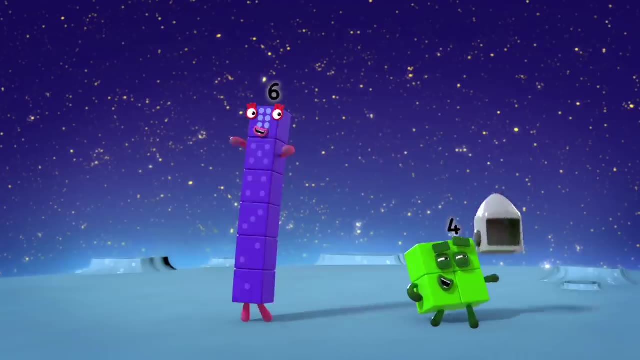 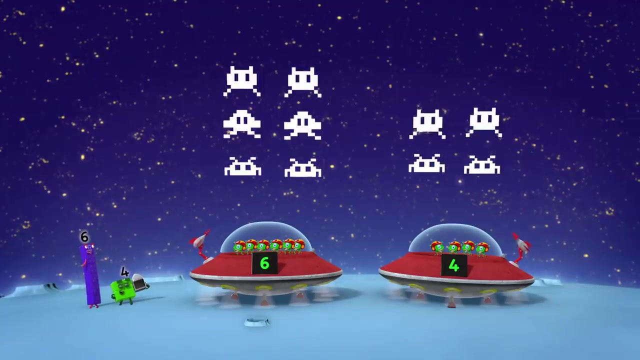 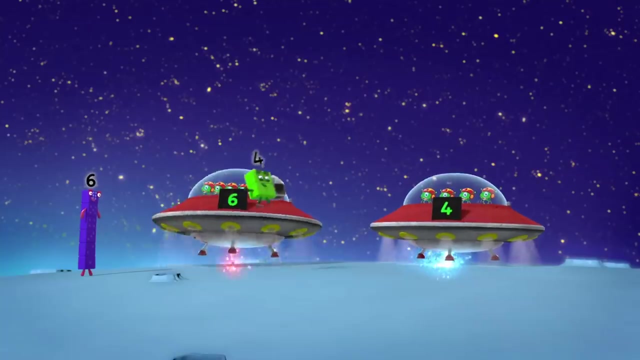 Ten equals Six plus four. We're on the moon. Six and four. We really couldn't ask for more. Let's play a game, Roll the dice. and Oh, That was so cool, Still too heavy, Oh, Oh. 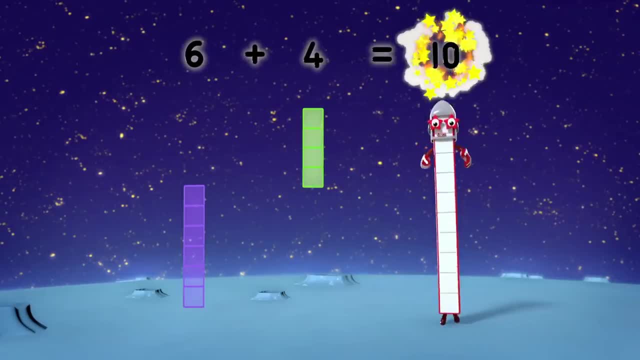 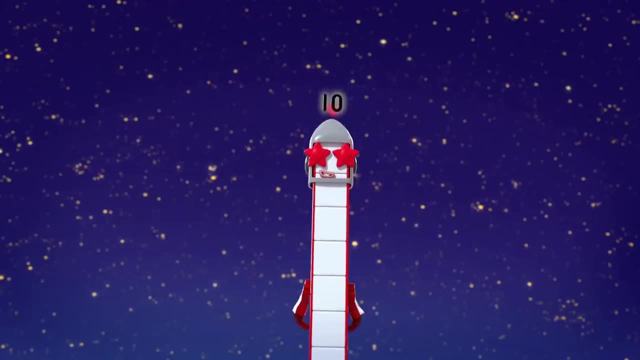 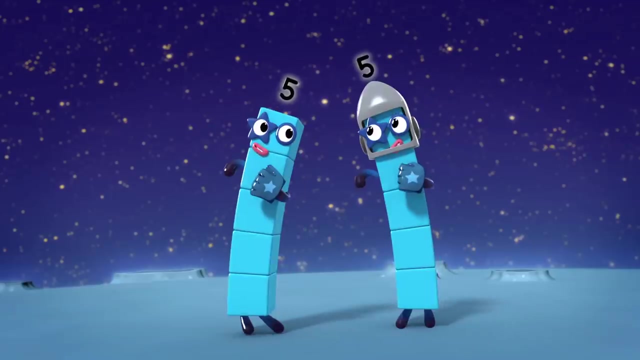 Six and four. Six plus four equals ten. Quick, before our visit ends, We've just got time for two more friends. Ten equals five plus five. We're on the moon. Five and five. It sure feels great to be alive. Let's give them a hand. 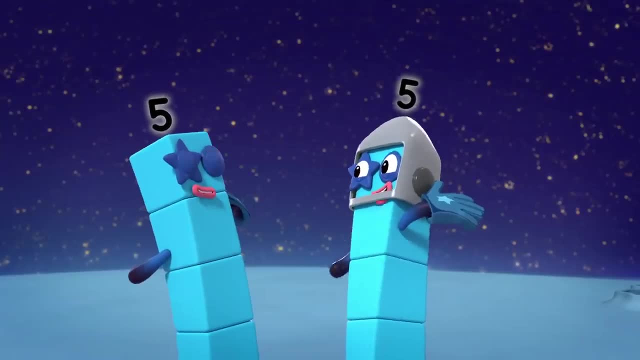 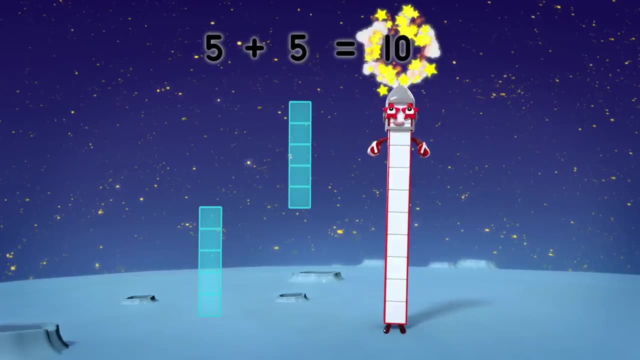 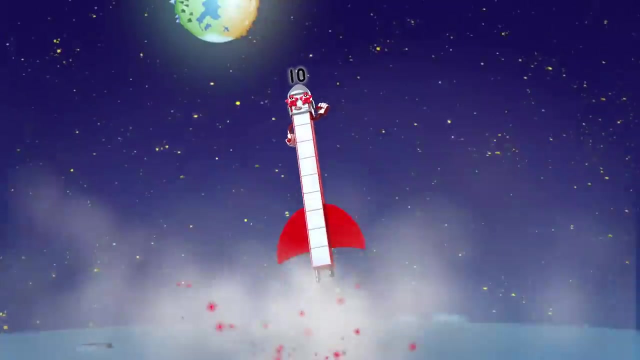 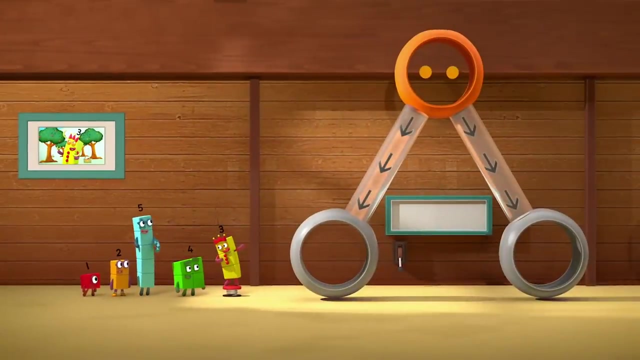 Ha-ha, High five, Come on. Five Plus five equals ten. The number blocks from one to ten went to the moon and home again, Welcome, welcome. welcome to my fantastic Fun Fruit Factory where we serve up fresh fruit all day. 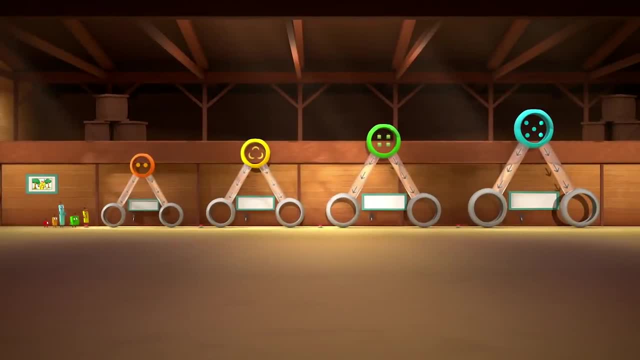 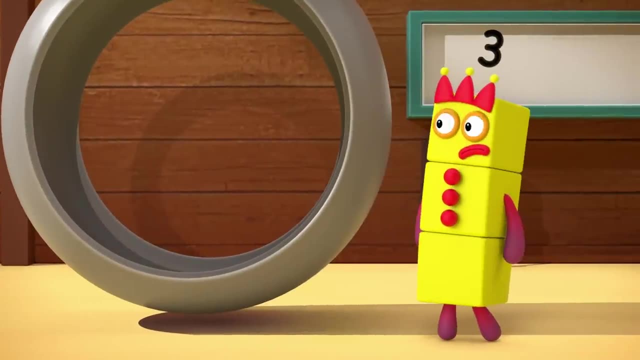 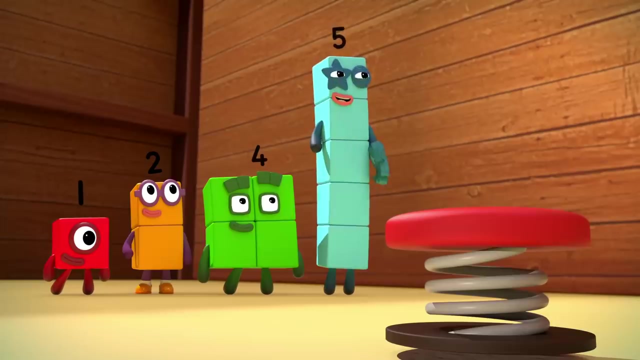 Ooh, Wow, How do they work? Oh, easy peasy, lemon squeezy. All right, I'll take a look. I guess I should make a contact语: Ooh, Ooh, Oh, I'm going somewhere. 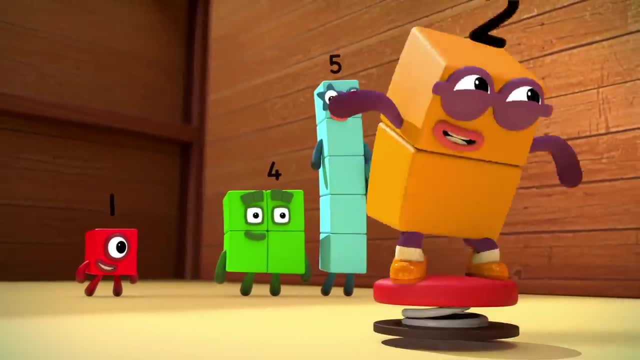 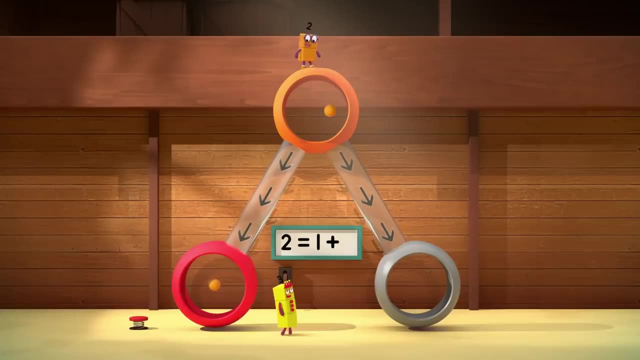 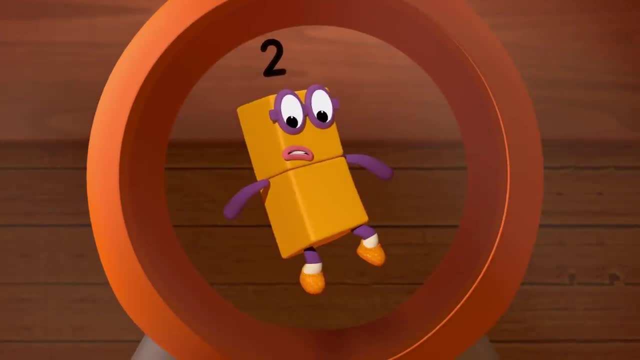 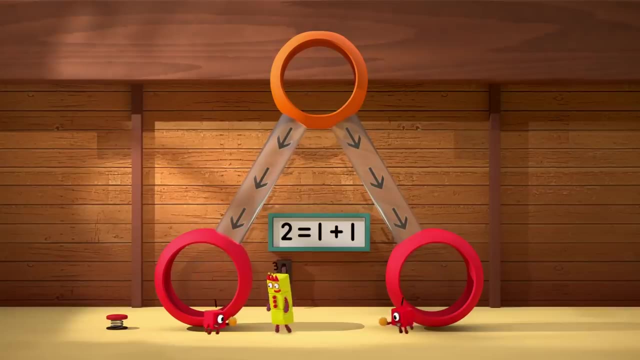 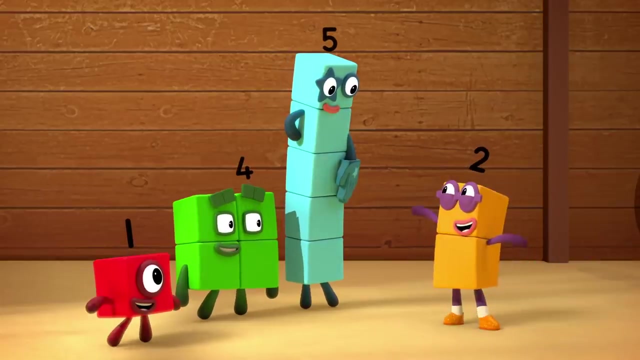 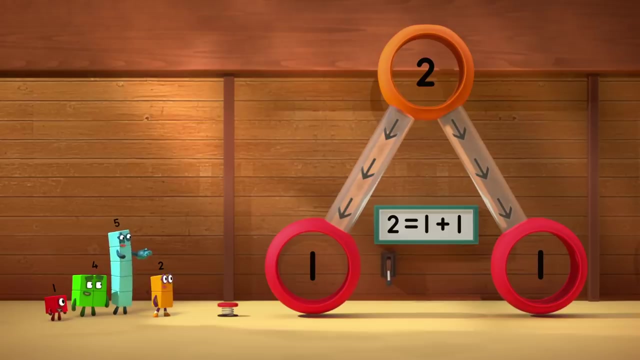 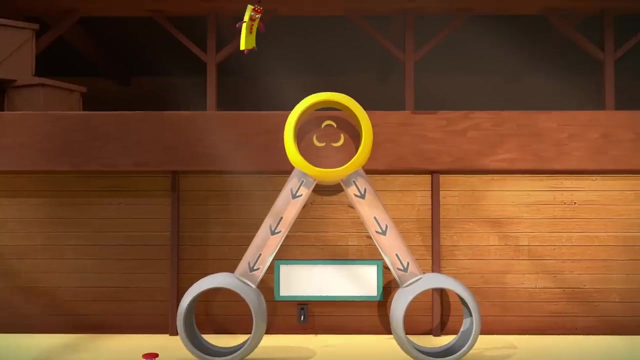 Come on. Two Equally, One Plus One. Yum Ta-da. Look. Two at the top splits into one and one at the bottom. I want fruit. It's my turn. Three equals one plus two. 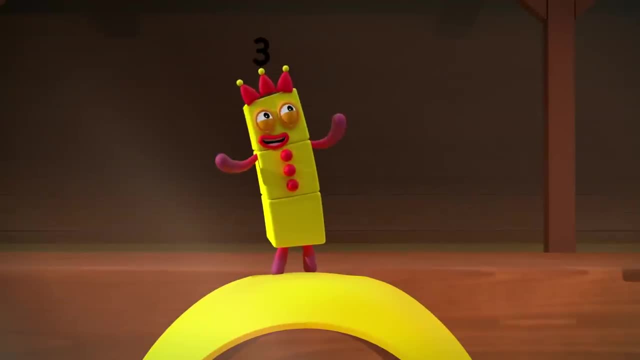 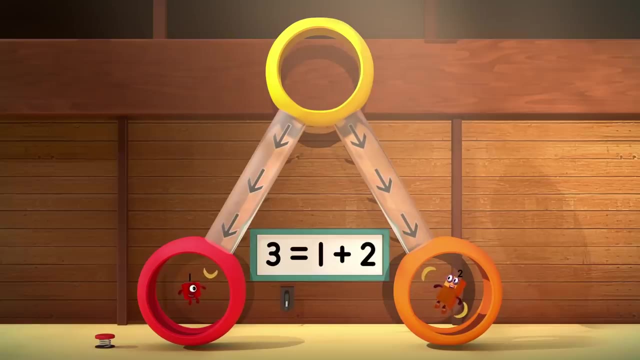 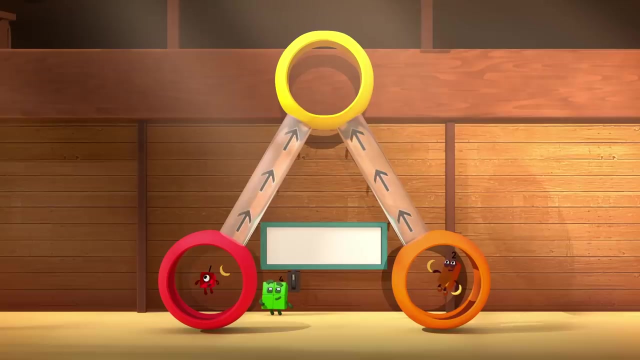 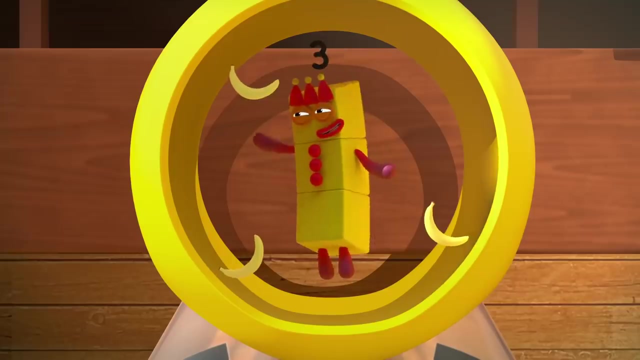 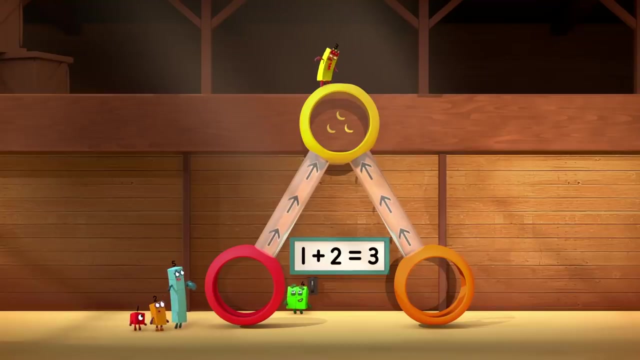 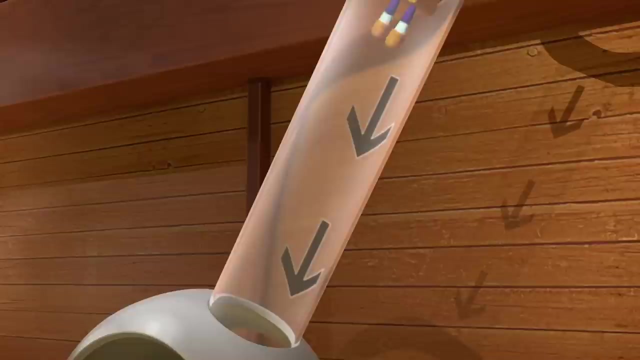 Yummy, yummy, yummy. Three equals one plus two. Oh, Where's three? Let's try this lever: One plus two equals three, Three. Oh, It works both ways. Hey, Those are mine. Three equals two plus one. 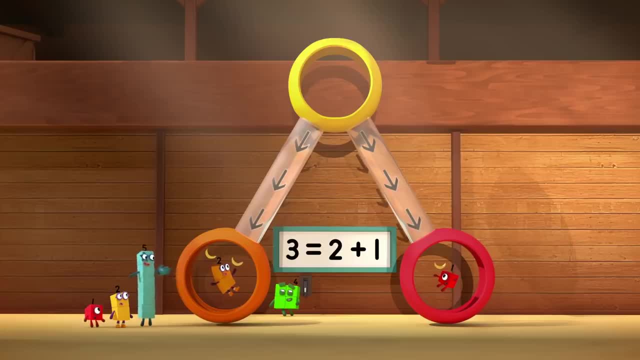 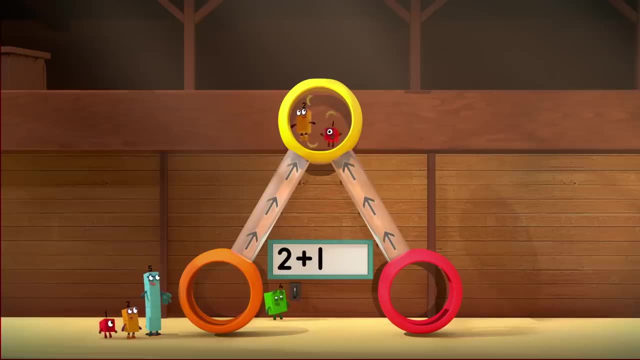 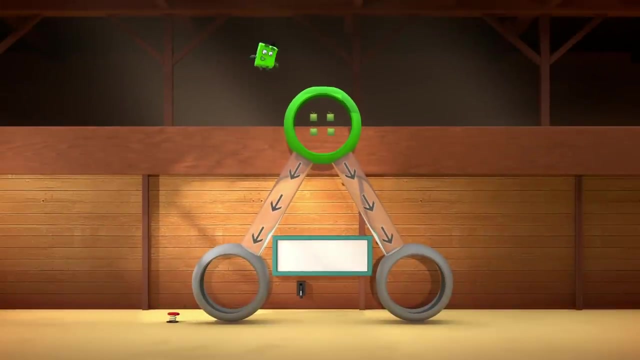 Now there's two over here and one over there, But three doesn't get her bananas again. Two plus one equals three, Three, Hey, I'm still hungry. Look, Apples Square apples. Four equals two plus two, Yum, yum. 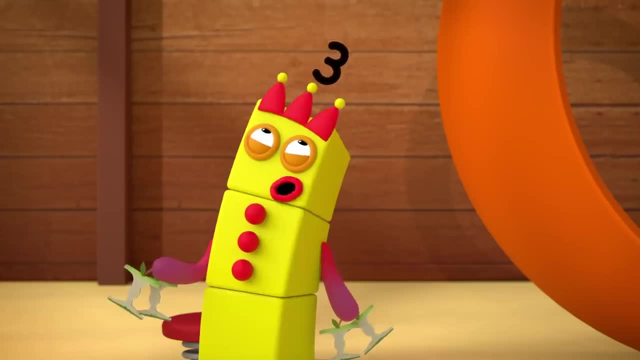 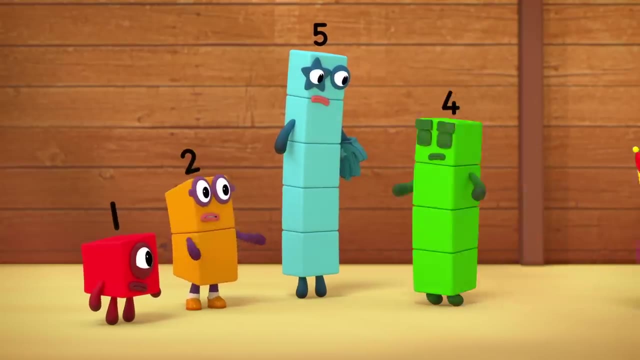 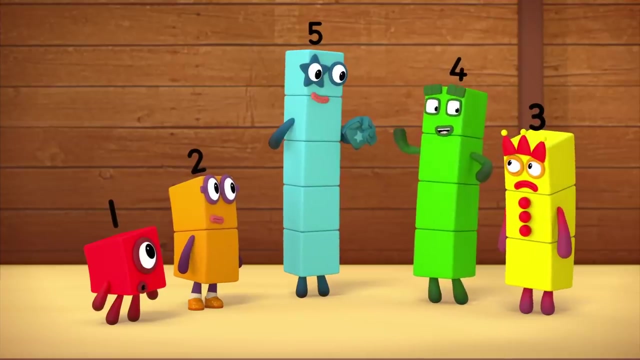 Yum, yum, No, no, no, you silly machines, Poor three. We need to find a way to make three apples come out. Look Four new apples at the top. I know how to make three, Here I go. 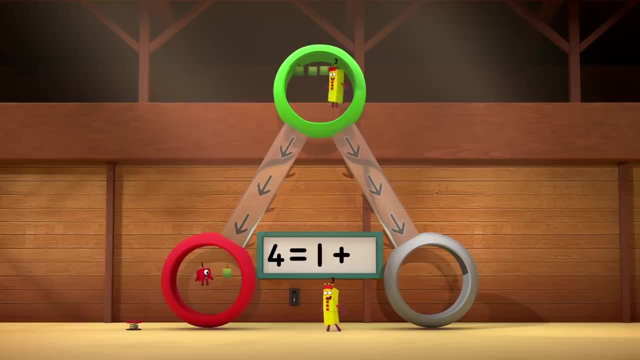 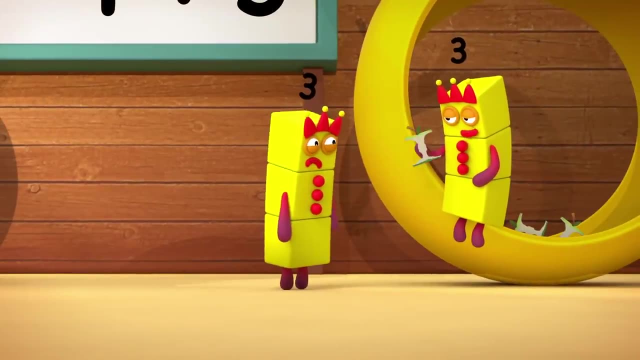 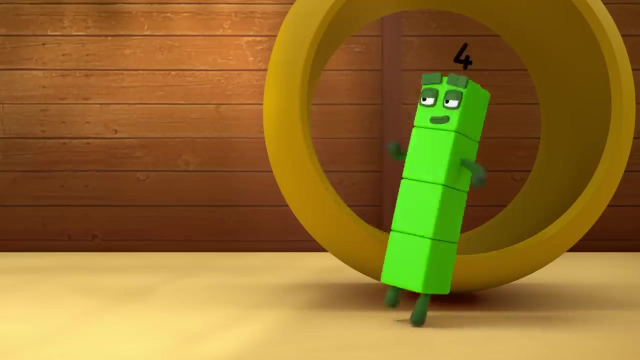 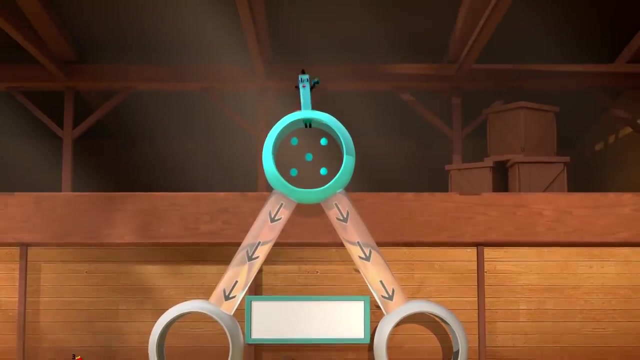 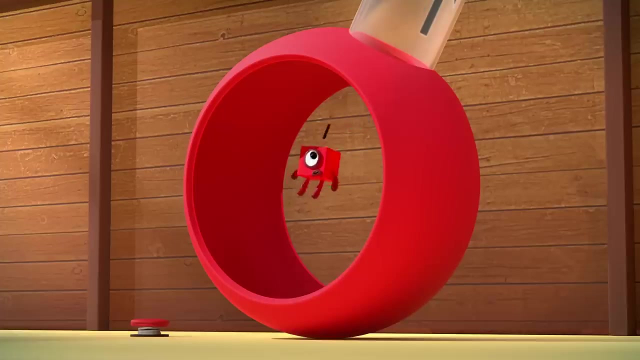 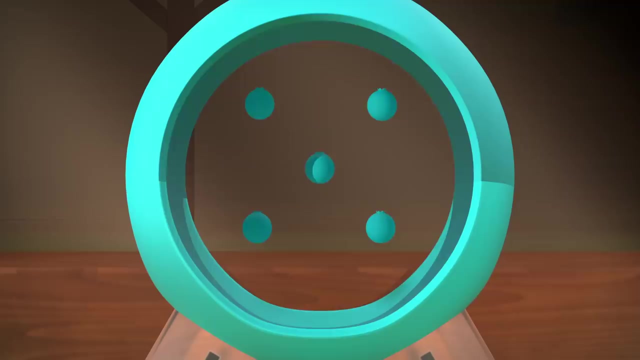 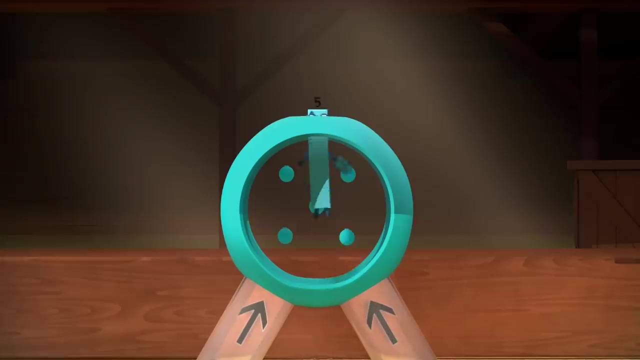 Four equals one plus three. Three, Yes, yes, yes, No, no, no, I won't front. Five equals one plus two. One plus four equals five. Five, Five equals four plus one. Four plus one equals five. 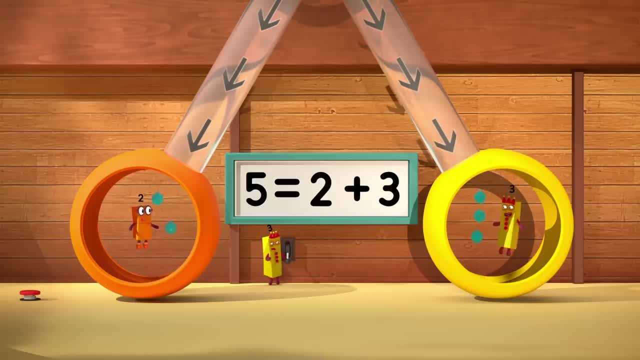 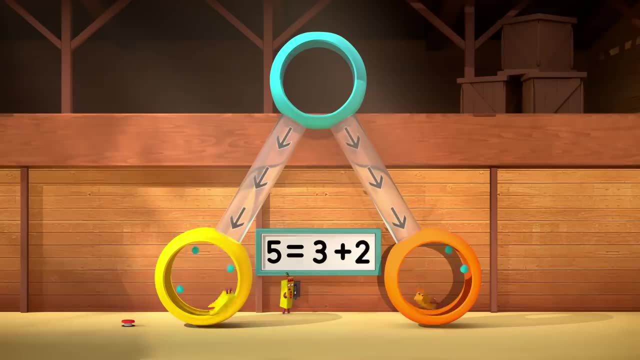 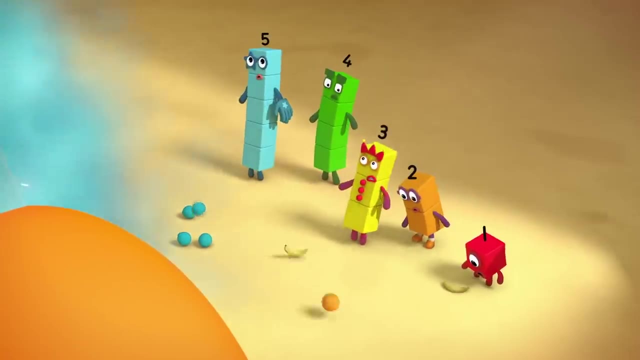 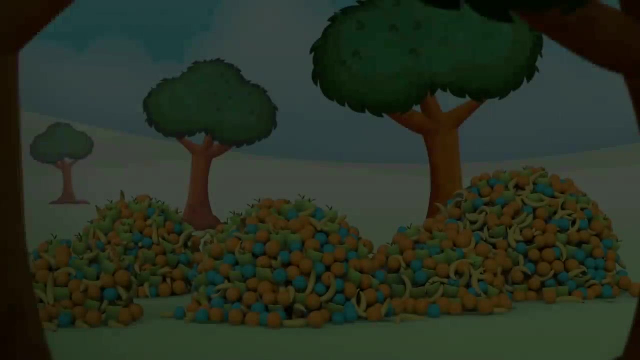 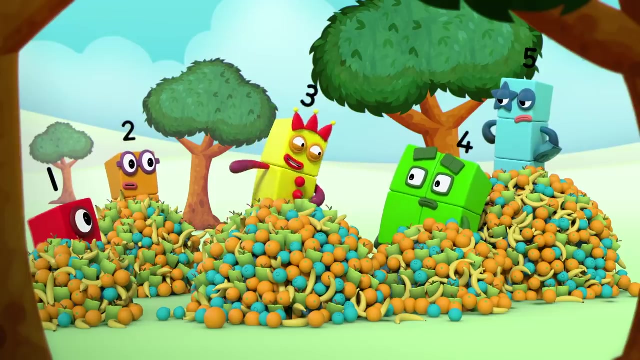 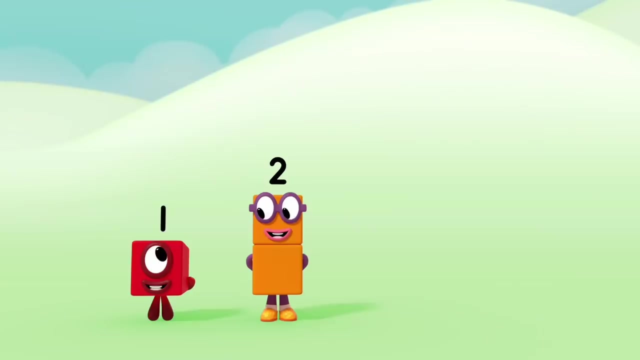 Five equals two plus three. Two plus three equals five. It's going far too fast. Five equals three plus four. One, two, three, Three. blue birds- I told you Easy peasy: lemon, squeezy Ow. One plus two equals three. 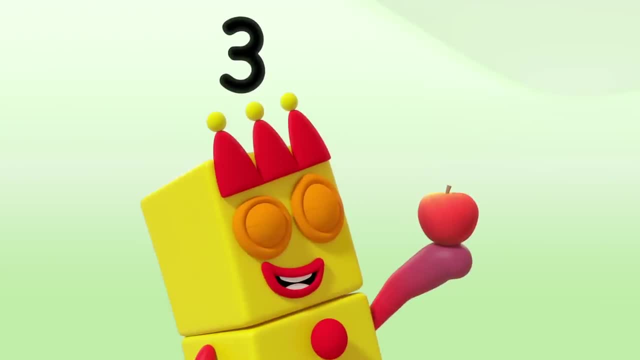 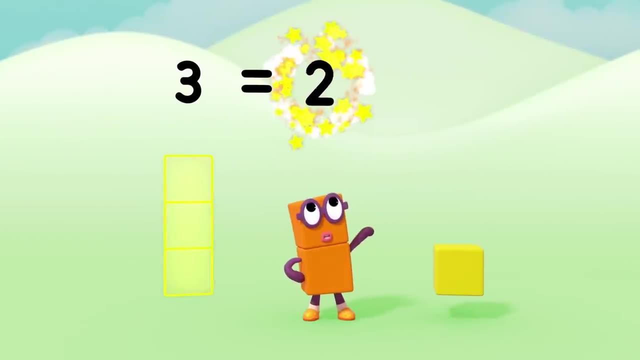 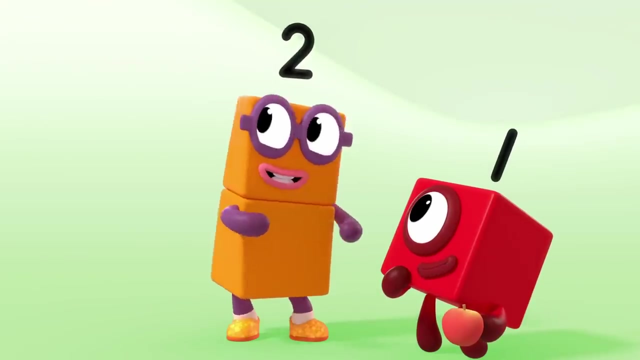 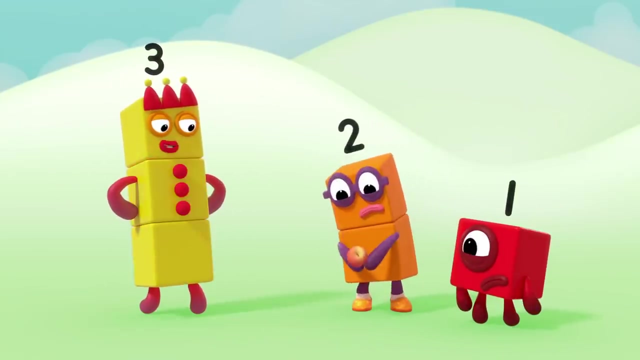 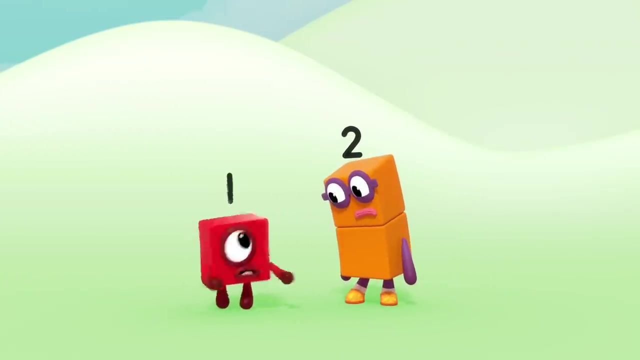 Three, One, two, three, Three equals Two plus one. Wow, But how Very good. You win best surprise. Three, One, two, three. Oh, that was the last one. Aww, Mmm Oh. 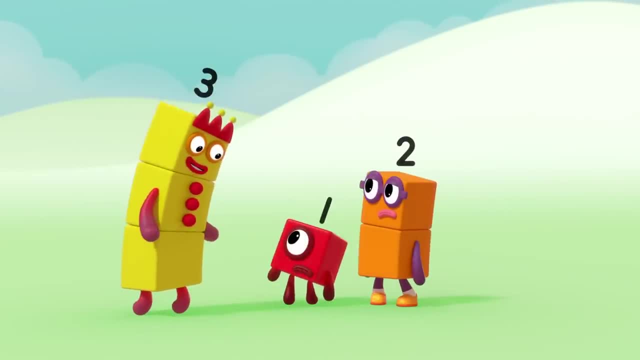 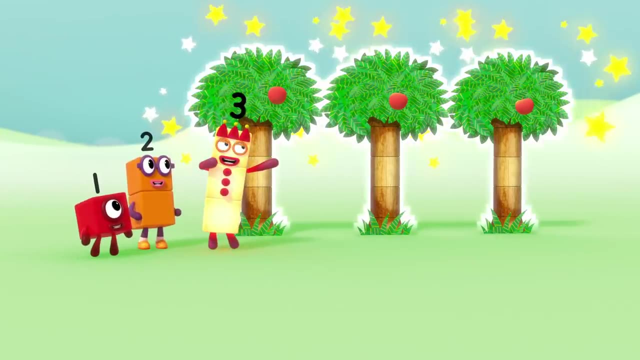 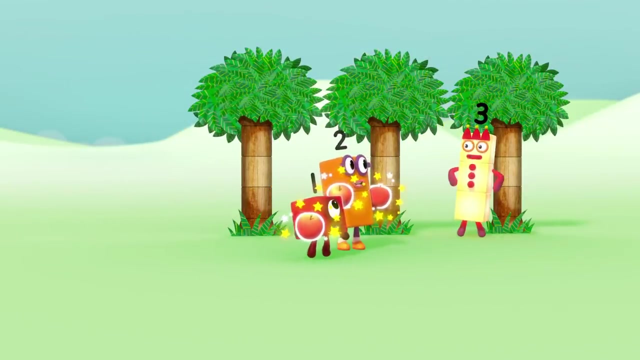 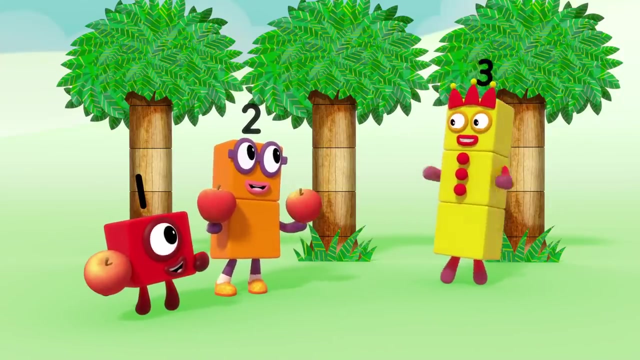 Don't be sad, Don't be mad, Be glad. One, two, three, Three trees With one, two, three, Three apples, One for me and two for you And two for me. I've already eaten three. 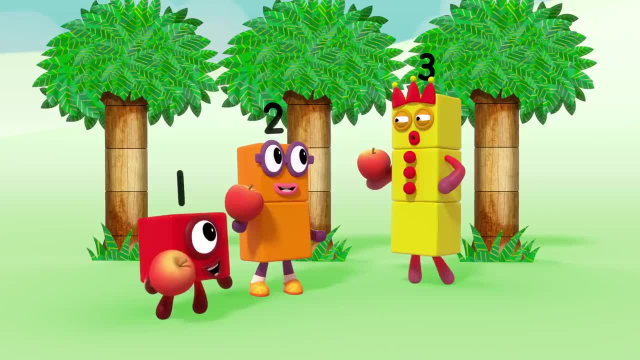 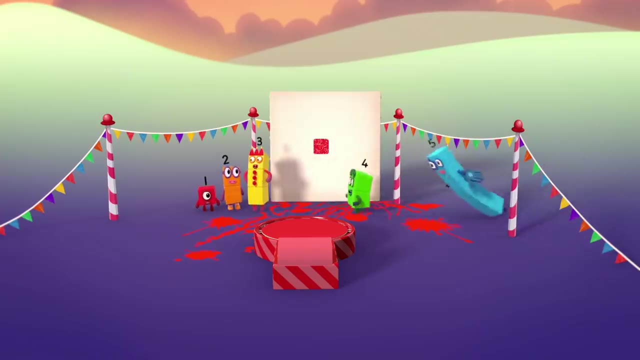 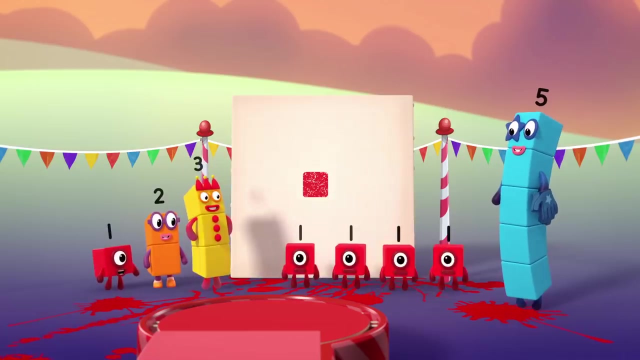 I don't mind sharing. Thank you Two. Now for my final trick. Let's make these apples vanish. One, two, three, Now, now. now You're forgetting something. One, two, three. Hey, One plus one plus one plus one equals four. 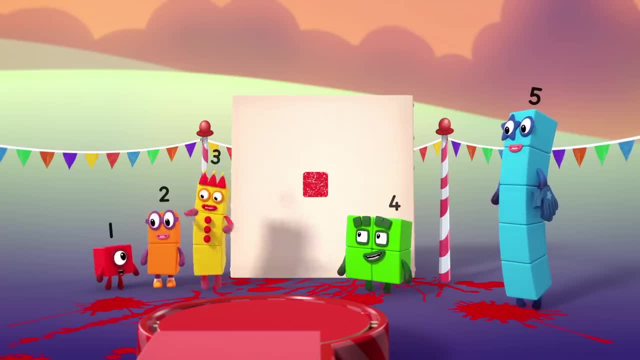 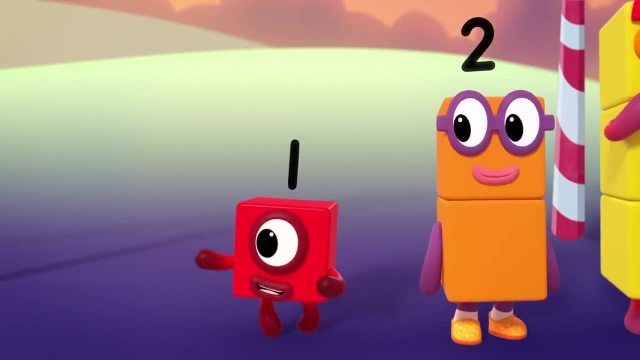 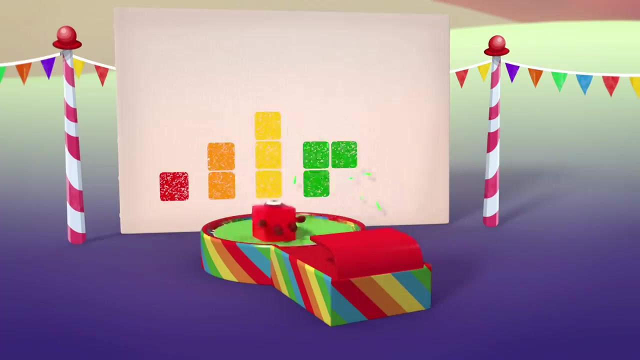 Every big shape is made up of lots of little ones, So lots of little ones can make every big shape. Look what I can do: Hooray, Hooray, Hooray, Hooray, Hooray, Hooray.